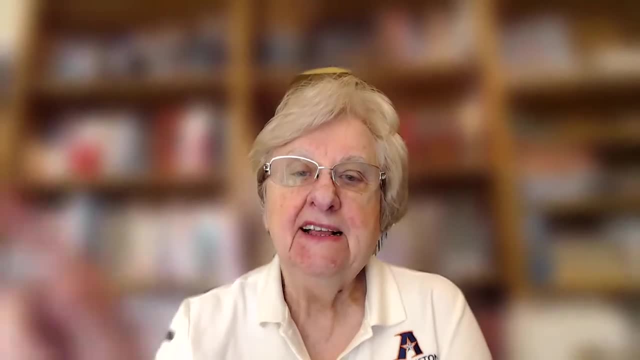 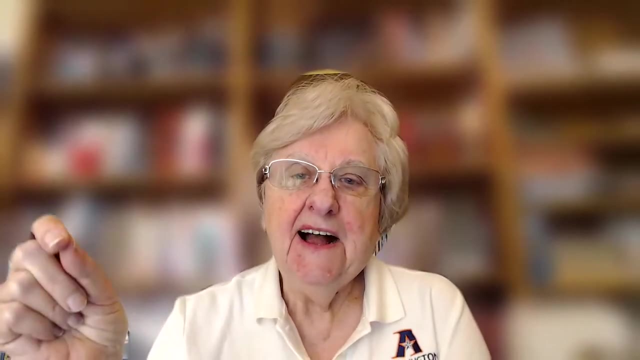 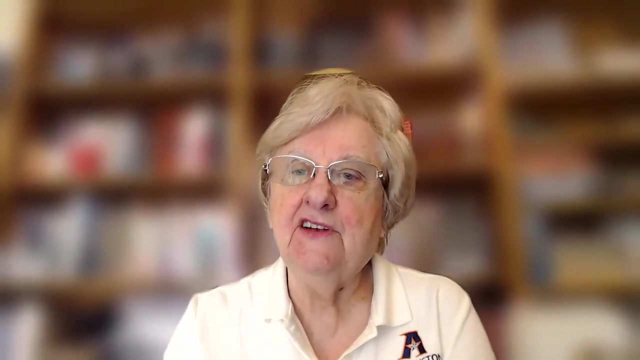 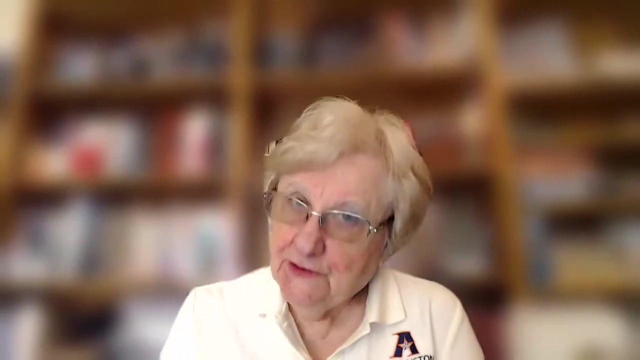 Available to you through Teams, and those questions will be dealt with after the presentation. The presentation is being recorded and it'll be available to all of us later on the YouTube page after today. So welcome to you. We believe that we have a number of our 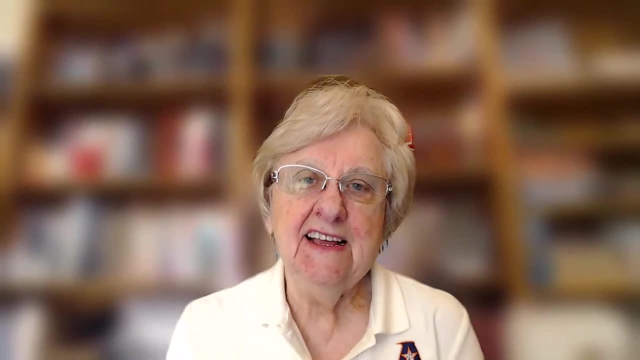 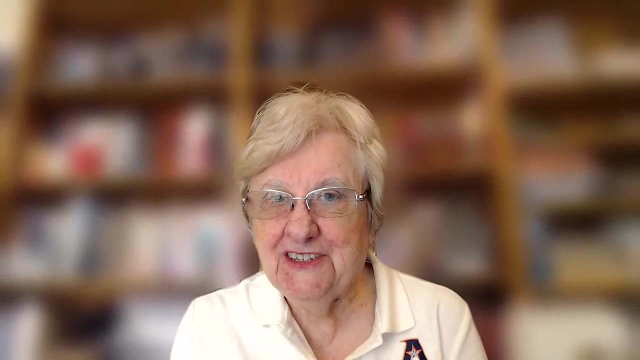 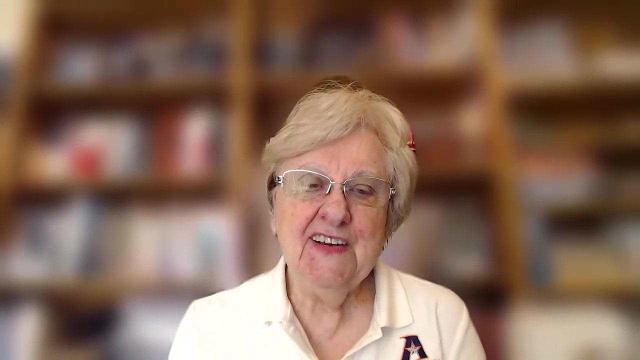 questions. We have a number of questions that we would like to answer Current UTA students, faculty staff, particularly the members of the American Nuclear Society student chapter, who is a very active group on campus, And we are very appreciative today of. 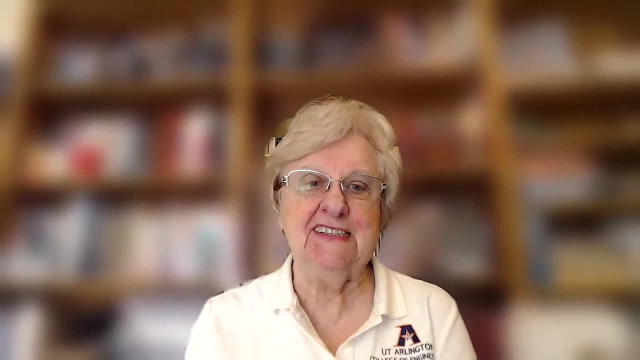 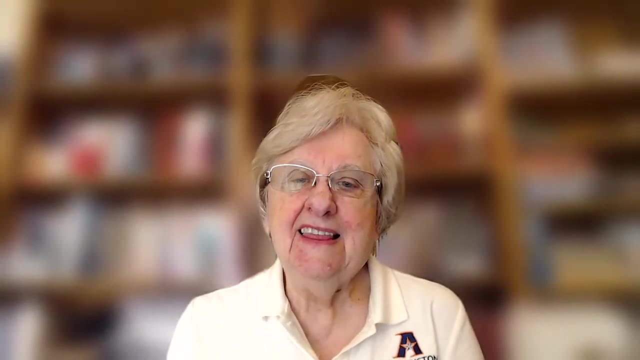 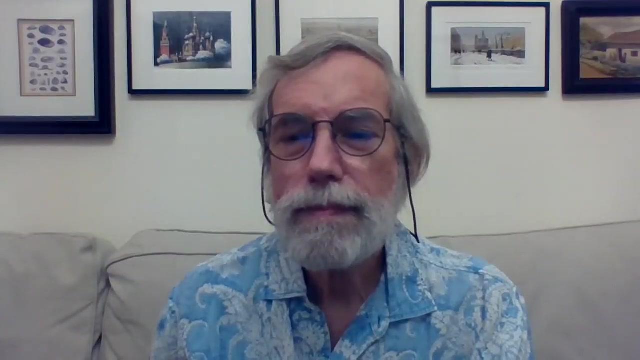 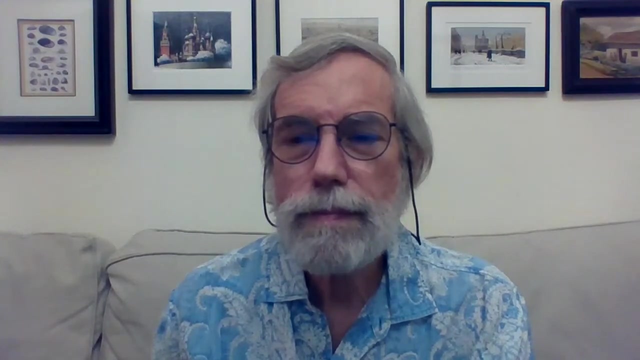 this opportunity to be part of the virtual brown bag series. So our presenter, David Graves, is the- or was, I guess, prior to retirement, the senior nuclear officer for safety in the International Atomic Energy Agency That is based in Vienna, and he is living in Vienna and is presenting today. 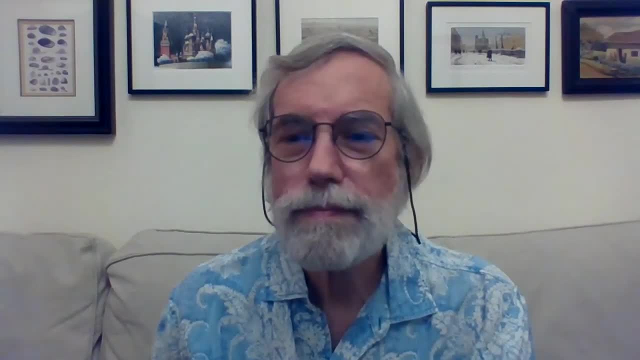 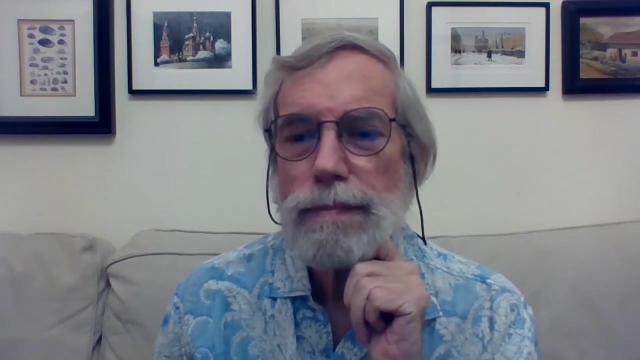 from there. Prior to his stint of eight years in the IAEA, he spent 24 years in the US Nuclear Regulatory Commission doing operator licensing and reactor inspections. The nice connection there is that Region 4 of the US Nuclear Regulatory Commission is based. 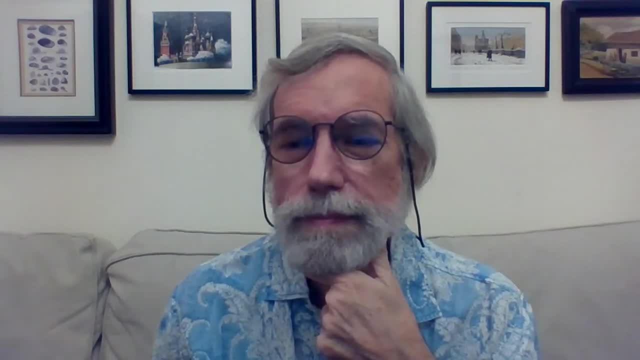 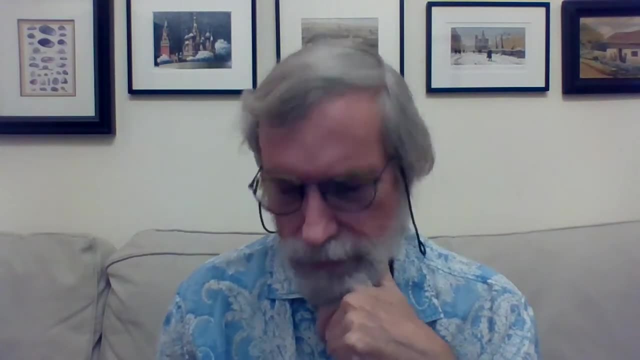 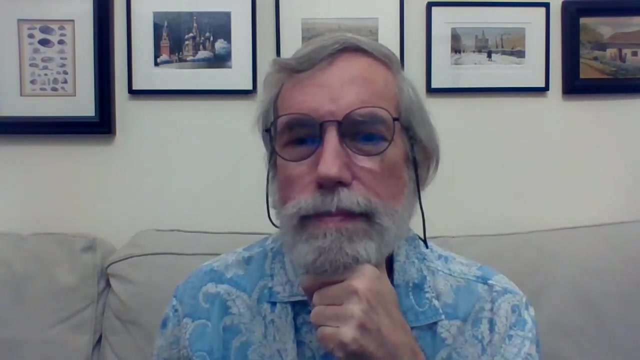 in Vienna That is based in Vienna, Arlington, Texas, So he really has a UTA connection that we are taking advantage of today. Prior to his time at the Nuclear Regulatory Commission, he was in reactor operations and training in a commercial nuclear facility, a DOE test reactor and US Navy submarine reactors. 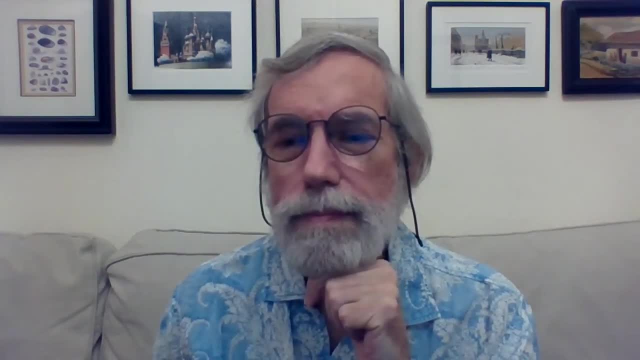 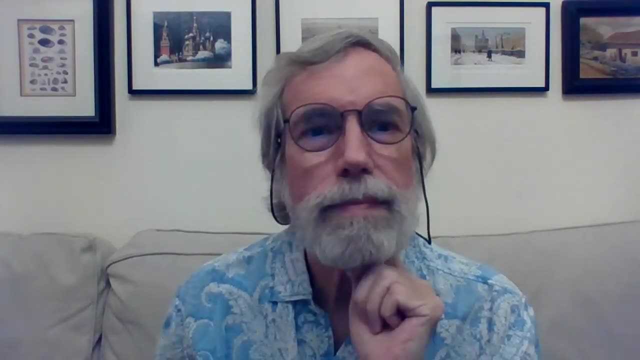 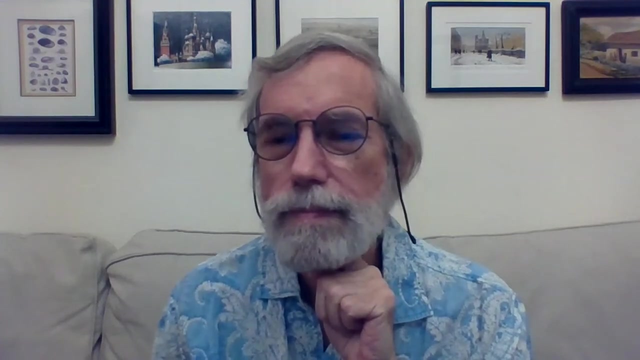 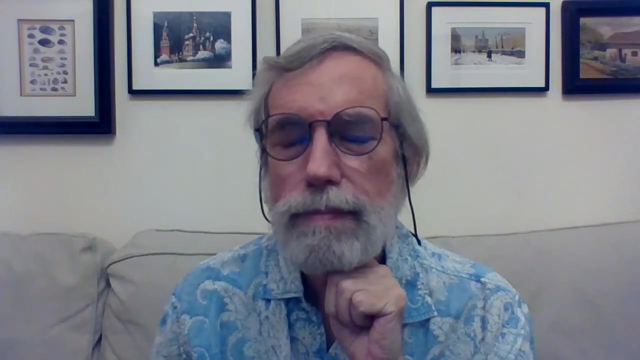 There was another nice Arlington connection in that David's wife Martha was director of outreach for the College of Engineering at UTA. So lots of reasons that we are very appreciative of David spending some time with us today to talk to us about the International Atomic Energy Agency. 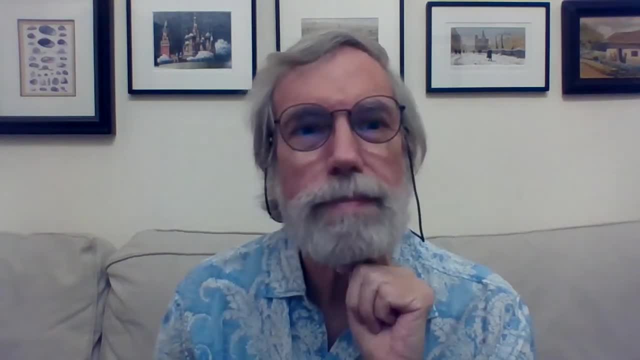 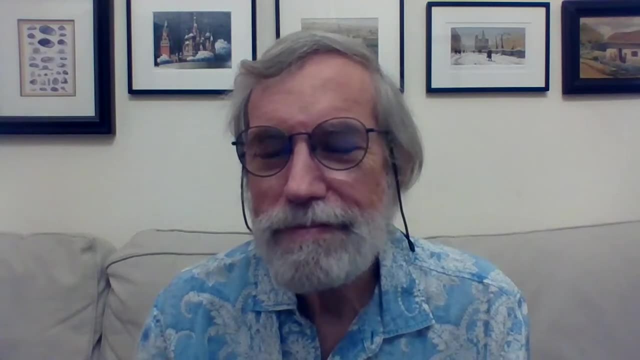 IAEA 101 is the name of the agency. This is his presentation. So, David, thank you so much for spending the time with us today, and we're really looking forward to what you have to tell us about IAEA. Let me just mention this is an 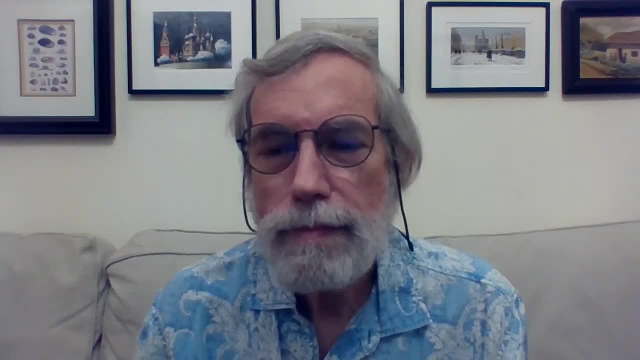 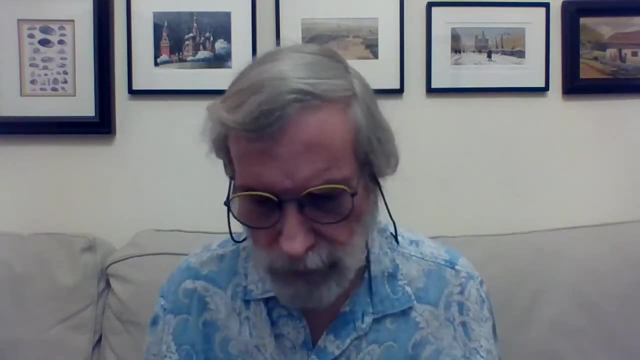 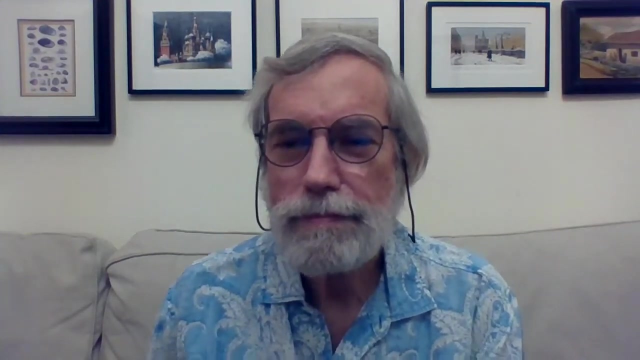 independent agency of the United Nations and is the world's central intergovernmental forum for scientific and technological cooperation in the nuclear field. So lots of relevant information about IAEA 101.. And thank you again, David, for spending time with us today. 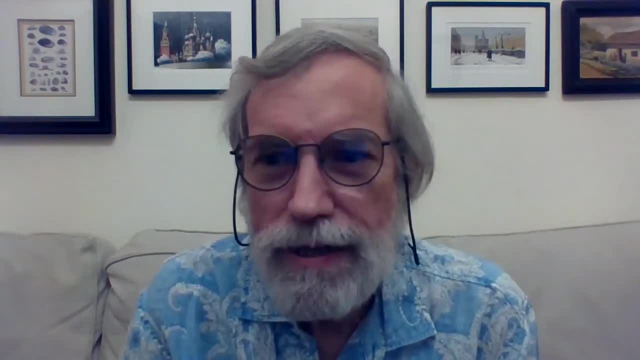 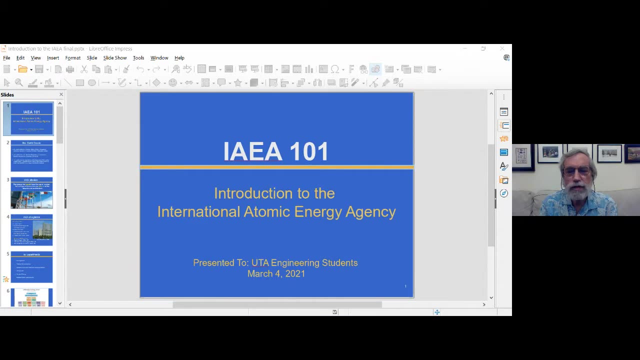 You're welcome, Lynn, and thank you very much for the introduction. As Lynn said, one of the things that I intend to cover today is kind of like a brief introduction to the IAEA, covering the organization and some of the activities that IAEA is involved in. 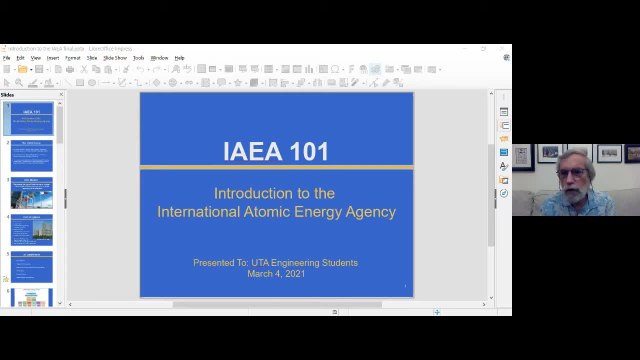 And as we go through the presentation, I'll start focusing more and more on my specific activities, what I did, and then, toward the end, I'll talk a little bit about the various employment opportunities at IAEA and different things that you can be involved in and how to get in touch with. 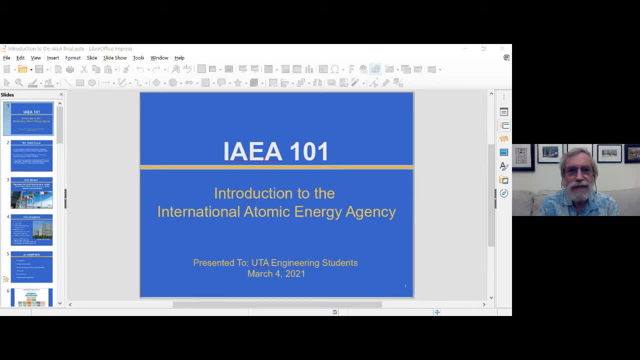 them. So, as Lynn said, I was with IAEA for a little over eight years and specifically I was in the regulatory activity section, which was a natural feed from being with the Nuclear Regulatory Commission for a couple of decades- My full time with the Nuclear Regulatory Commission. I was in the Arlington office. 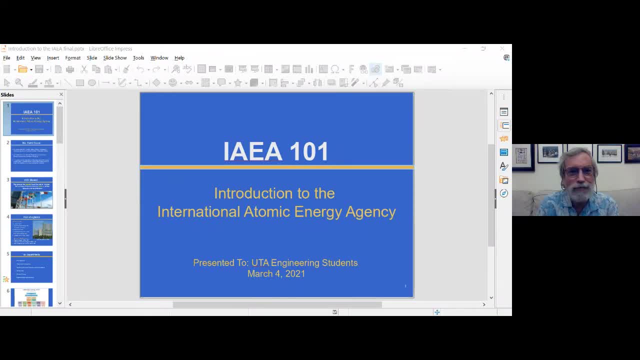 in the Region 4 office just down the ways from you there, The various operations facilities at Westinghouse, the pressurized water reactor under construction in South Carolina and the Department of Energy test reactor at the Idaho National Laboratory- At the time it was Idaho National- 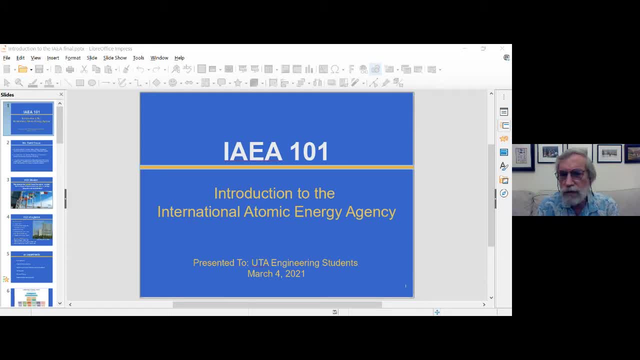 Engineering Laboratory and specifically it was the Loss of Fluid Test Reactor where we conducted loss of coolant accident experiments on a functional pressurized water reactor. And then I spent some time as a reactor operator on board Navy submarine operating reactors and also as an instructor at the nuclear training facility for the US Navy in Idaho. 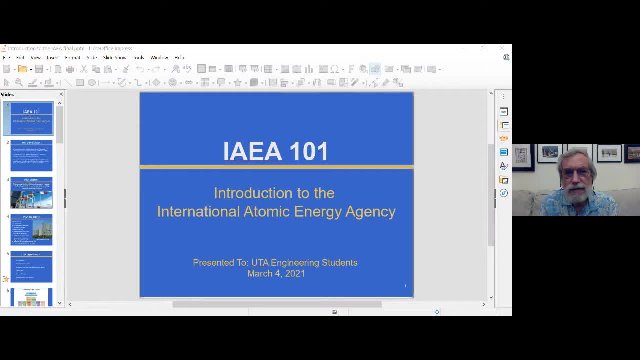 The general mission of the IAEA is maximizing the benefit from the use of nuclear technology while minimizing the risk and safety, security and proliferation. As we go through this, you'll see that there are a number of different activities, both from a promotional side for the use of 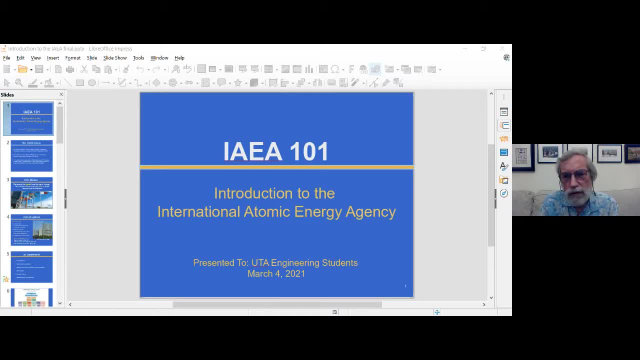 nuclear energy and radioactive materials, and also the safety side, as well as trying to limit the nuclear proliferation of nuclear materials from a weapons standpoint. Just some general information about IAEA. It was founded in 1957 as an offshoot of a speech that. 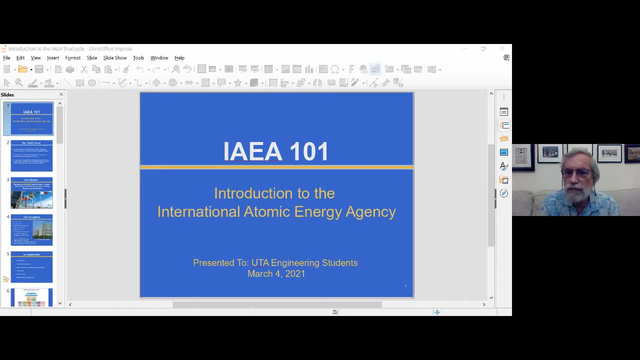 President Eisenhower gave regarding the peaceful use of nuclear weapons in the United States. It was developed by the Texas Civil Engineering Association, the US Navy and the Texas Federal Air Force. It was created by President Eisenhower to be used for the use of nuclear 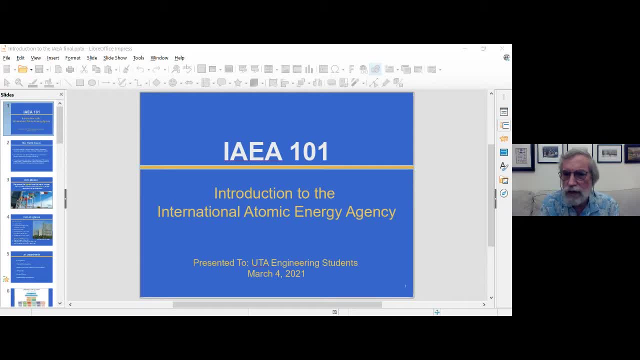 power, the Atoms for Peace Program. There are currently 172 member states of IAEA And, as Lynn said, it's an independent agency of the United Nations. So just being a member of the United Nations does not automatically make you a member of IAEA. It has to be applied for separately. 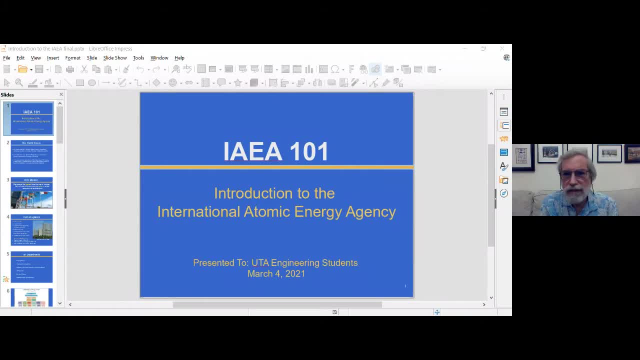 and accepted. The headquarters are in Vienna. and that photo. there is a picture of the headquarters building complex. It's called the Vienna International Center, Even though the headquarters are in Vienna. there are three different scientific laboratories and research centers that are associated with IAEA. 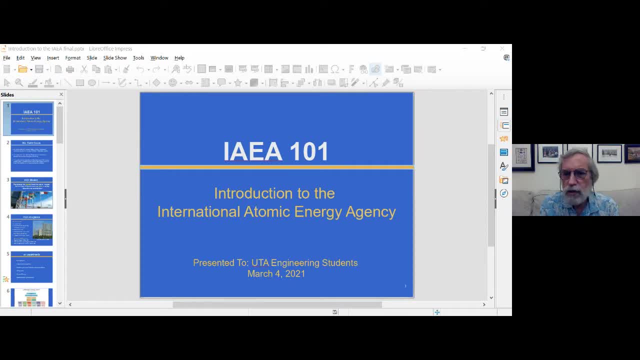 In Austria, in a little town called Seibersdorf, there's a laboratory complex where they do a lot of analysis, sample analysis and things like that. In Monaco there is an ecological and environmental monitoring laboratory, And in Italy, at a university in Trieste, Italy, there's a physics research center that IAEA has a cooperative agreement with. 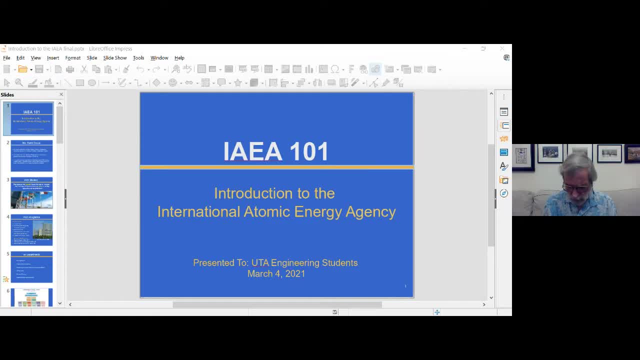 David, your slides are not advancing. I think you're on maybe the second or third slide already. Oh yes, It's not advancing, David, if you will just use your mouse to click over on that left-hand column, the small slides on the left-hand side. There we go. 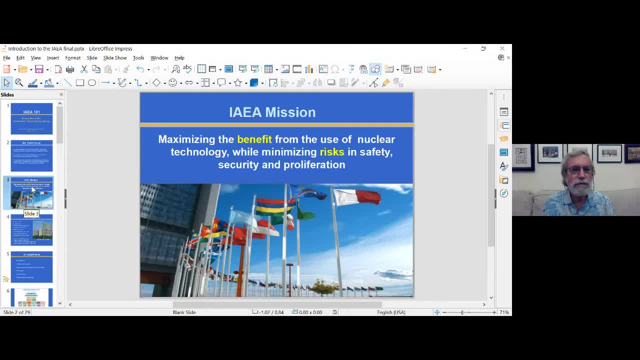 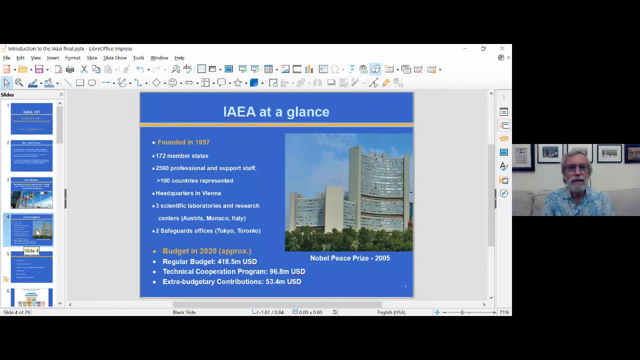 There we go, Got it, Thank you, Okay. So just use those. Yeah, let's do that at this point. That's good. Okay, I won't go through the same information again there, but I'll pick up at the three scientific laboratories. 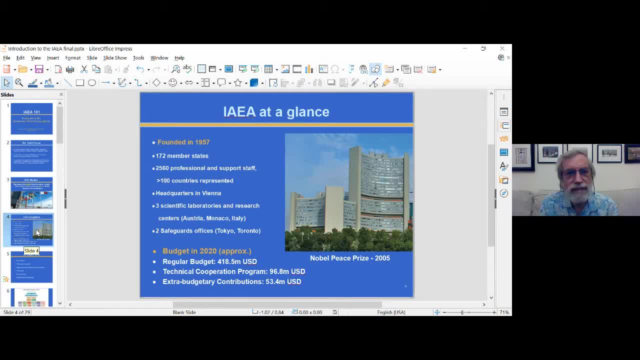 Seibersdorf, Austria, Monaco and Trieste, Italy. There are two remote safeguards offices, which we'll talk a little more about safeguards later. There's one in Tokyo and one in Toronto. From a money standpoint, obviously, nothing functions very well without money, but the budget in 2020 was approximately $418 million for the regular budget. 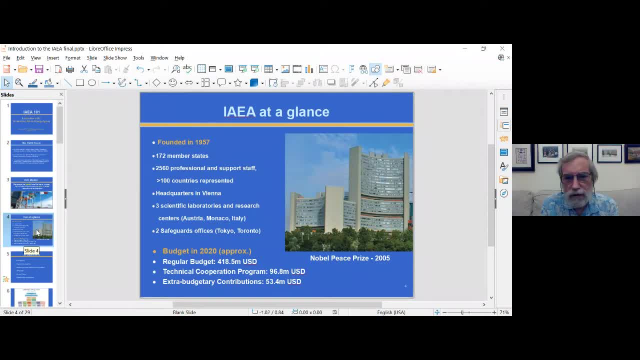 Technical cooperation was $96 million. Okay, There's a little over $96 million, and extra budgetary contributions are a little over $53 million. Where that money comes from, it's all by donations from the member states. Regular budget covers the normal functioning of the agency. 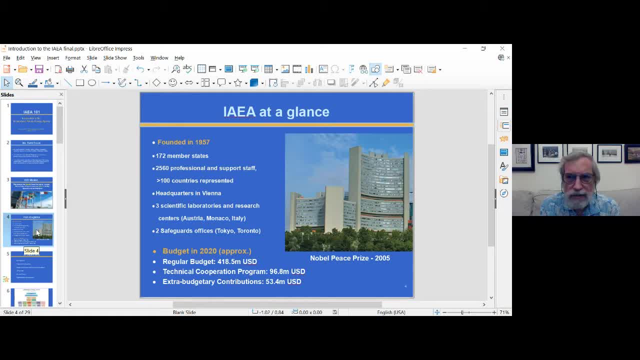 Technical cooperation budget provides funding and assistance to, I would say, developing countries, the lesser developed countries that need assistance with various aspects of nuclear power- Okay, The use of nuclear and radiological material, And that assistance is provided again by donations from member states that can afford the donations. 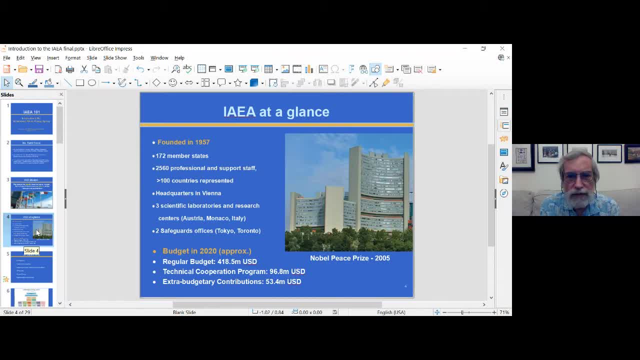 And we'll talk a little more about the technical cooperation program in a little bit- And extra budgetary contributions are funds that are contributed by member states that basically have strings attached. They donate money for specific purposes or for specific functions or programs where they can contribute. 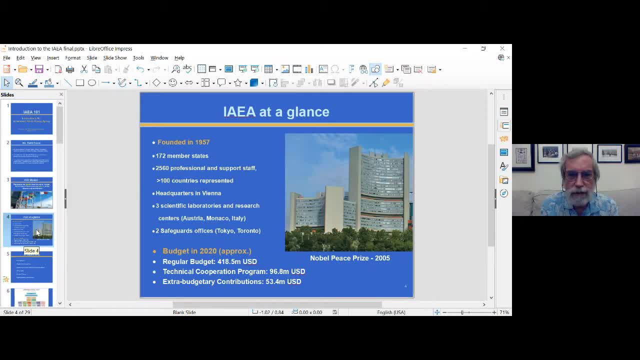 Okay, Thank you, Thank you, And they direct what they want the money to go for. Also, as an aside, right under the photograph there you see the Nobel Peace Prize was awarded to the IAEA in 2005.. It was primarily for their work with the weapons inspectors in Iraq from a couple of years before that. 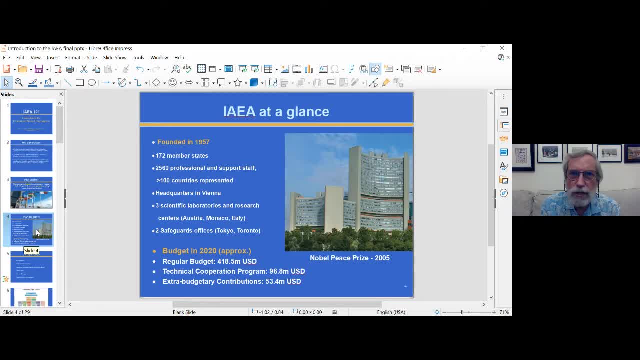 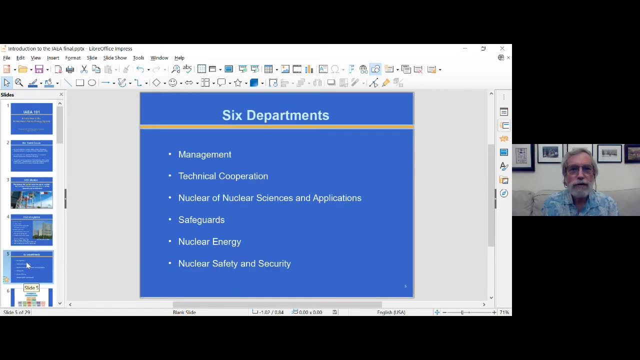 That prize was divided halfway to the director general at the time, which was Mohammad Al-Varadai, and half to the staff of IAEA. Thank you just missed out on the Nobel Prize. I got there in 2006, so so be it. there are six. 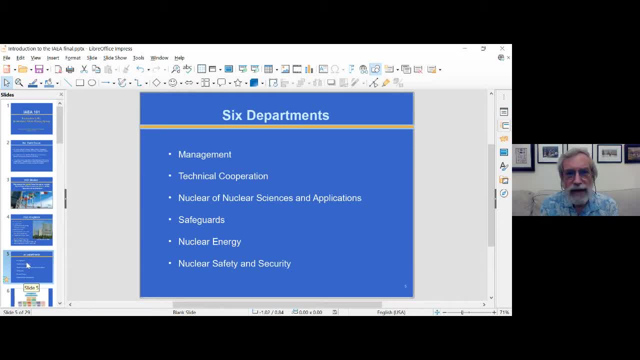 different departments in IAEA. there's the Department of Management, which is the administrative section that covers HR, budget, visa sections, things like that. the technical cooperation department is the department that is the bridge between developing member states and the technical departments of IAEA. they perform the administrative functions and program planning that member states need. 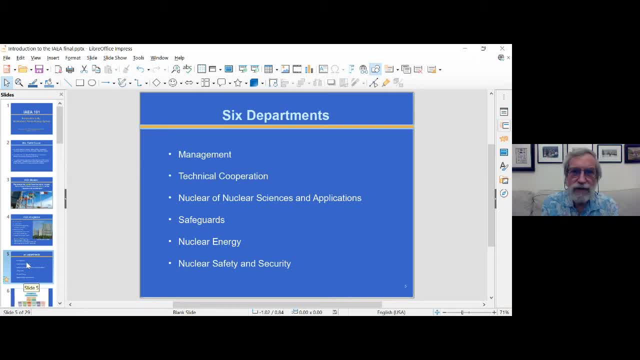 and coordinate that with the technical staff in IAEA to ensure it, to ensure that the projects get accomplished. the nuclear sciences and applications is another department that deals with more specific and important projects are located here at the IAEA of business specific uses of nuclear applications. 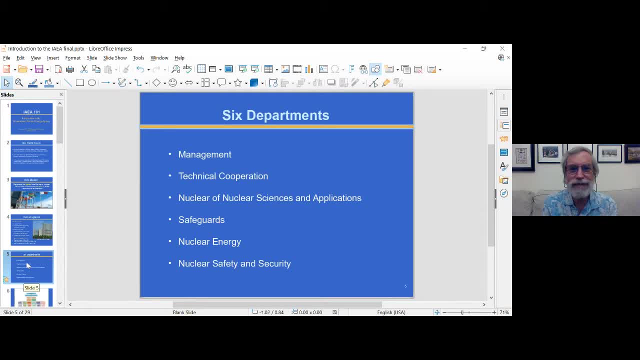 Well, there's that typo Should be Department of Nuclear Sciences and Applications. Sorry, Safeguards. Whenever you hear in the press when they talk about the nuclear watchdogs, that's usually the safeguards inspectors they're talking about. Safeguards is the department that is concerned. 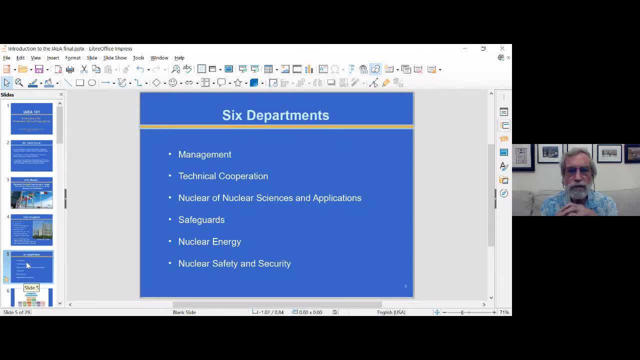 with the nonproliferation of nuclear weapons. So they're the ones that go out and do the weapons inspections, accounting for nuclear materials, things like that. So they are the ones that more or less you hear about in the press most of the time. 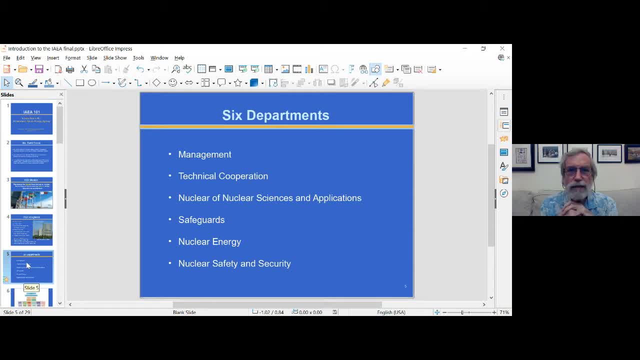 Nuclear Energy is a department that is primarily concerned with assisting member states with the development of nuclear energy. They are primarily on the development side to assist member states with the promotion and development of nuclear energy, And it's usually nuclear production and the development of nuclear power plants. 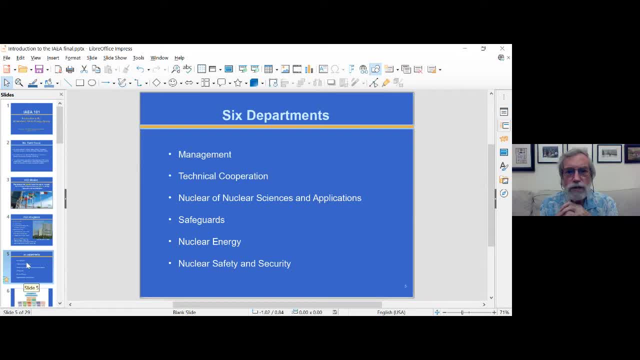 nuclear waste, that sort of activity. Nuclear Safety and Security: That department deals again with nuclear safety issues: Nuclear Safety, Emergency Preparedness, Safety and Security of Radioactive Sources, as well as the security of radioactive material And from the nuclear safety side. 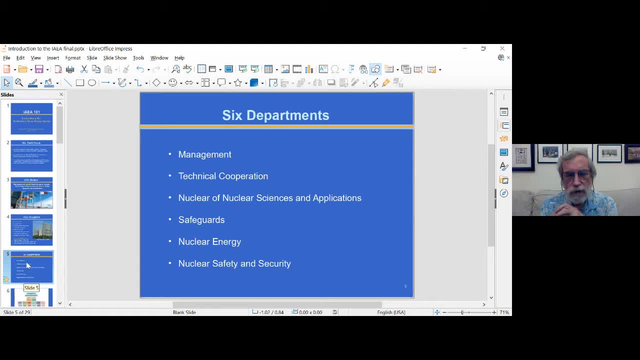 it doesn't just include nuclear power plants and things like that. It also includes nuclear or radioactive sources. There are only a limited number of countries that have nuclear power plants. Almost every country has some use for radioactive sources, whether it's medical uses, industrial uses. 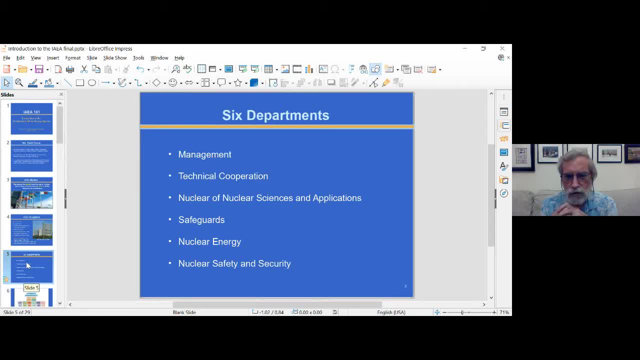 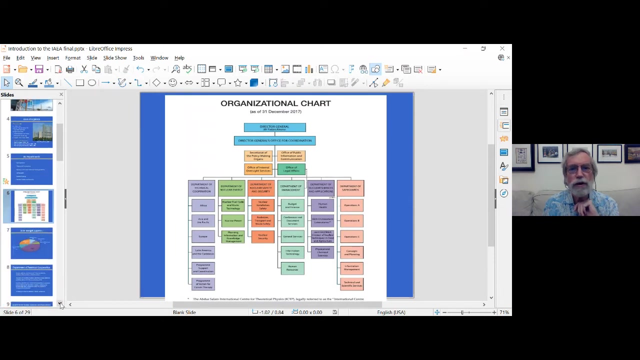 radiography, sterilization of foods. There are all kinds of activities that use radioactive materials And this department is concerned with the safety of that nuclear material as well as radiation protection safety. This is a general organization chart for the IAEA. It's pretty busy but it covers the 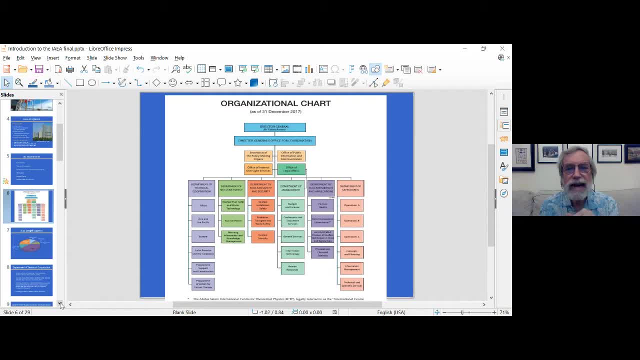 just shows the six main departments there and how they're broken up. Each one of the departments has a number of different divisions associated with it, And I was in the Department of Nuclear Safety and Security in the Nuclear Installation Safety, which had a number of sections in it. 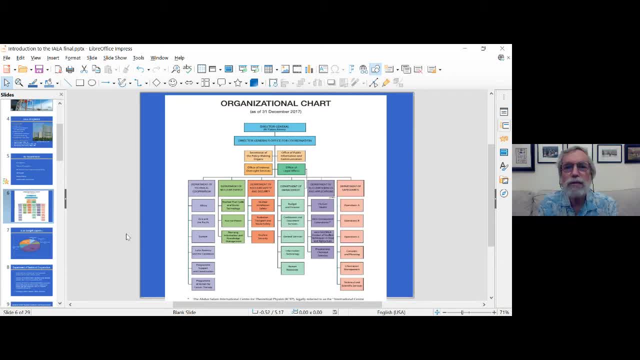 of which regulatory activities was one of them. One change on this organization chart: it shows the Director General as Mr Romano. Mr Romano passed away a year and a half ago, or something like that, And he's been replaced by Mr Rafael. 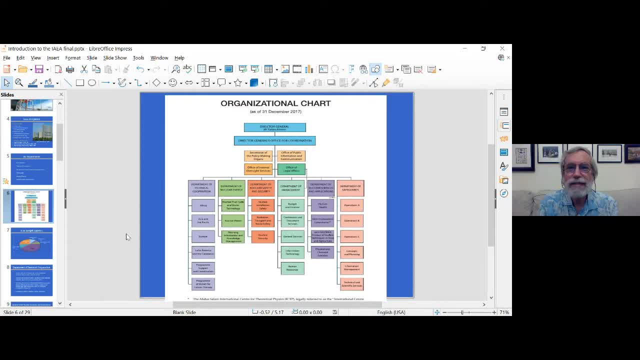 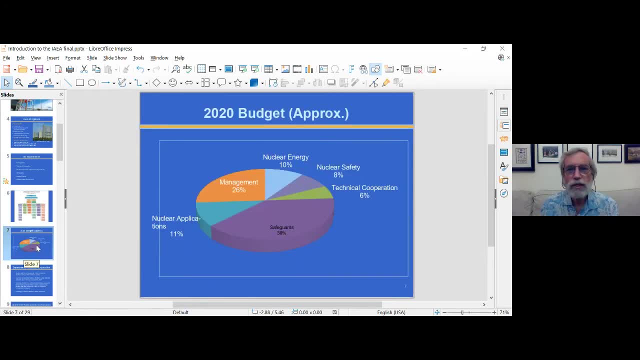 from Argentina And so he was just confirmed here within the last year or so. And the distribution of the budget, you can see that Safeguards has the lion's share of the budget. They do a lot of traveling. They go to all sorts of countries, you know, doing these nuclear inspections to ensure that nuclear materials are not diverted. 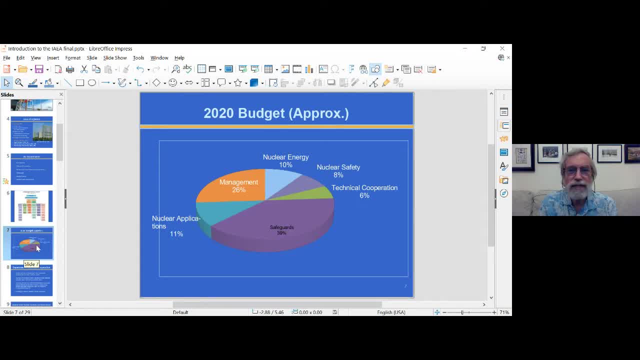 For weapons use or anything like that. So they comprise the biggest part of the IAEA's budget. And then you can see the other ones there: technical cooperation- six percent, nuclear safety eight percent, energy 10 percent, applications- 11 percent and admin management 26 percent. 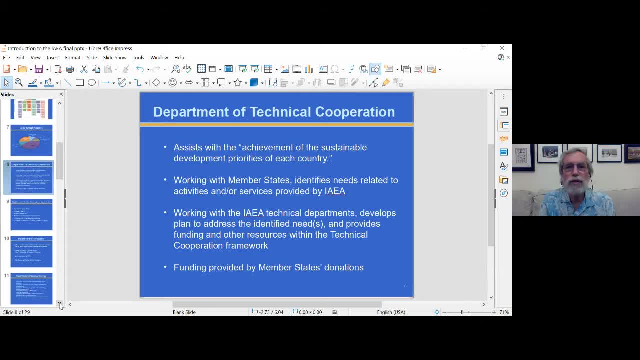 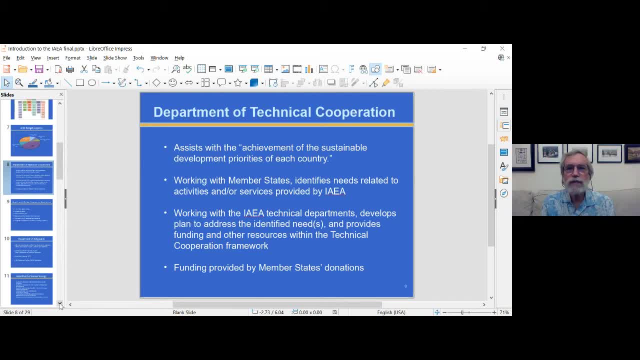 The Department of Technical Cooperation. they assist with the achievement of the sustainable development priorities of each country, And what they do is is working with the member states. member states discuss with IAEA what their needs are related to specific activities or services that we, that we could have, could help them with. 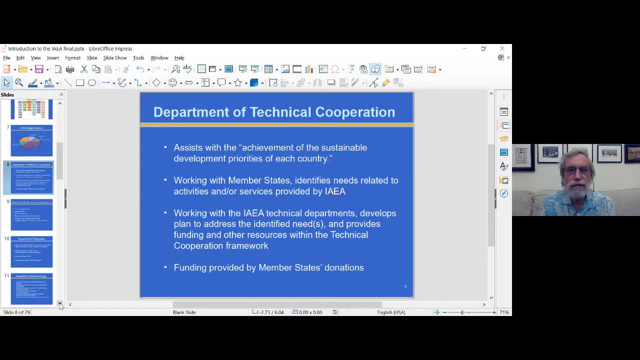 We come to. we would come to agreement with a member state on what what support they needed And then the technical cooperation group, along with the member state, would work with IAEA technical departments and they would develop plans and programs to address those identified needs. and those activities would be accomplished by IAEA providing funding, funding and other technical resources as necessary within the, within the framework or whatever was allowed by IAEA. 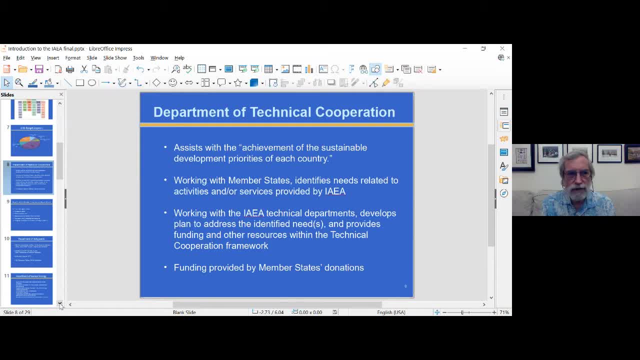 And this. this could be in the way of training, It could be in the way of material support, It could be equipment. There are lots of different activities. It just depends on what the member states It's needed at any particular time and also, as I mentioned earlier, the funding was provided by member states donations. 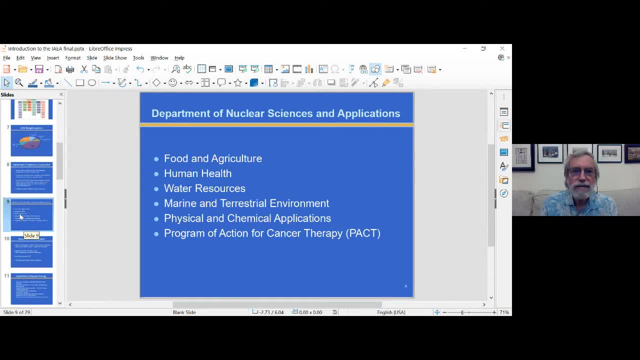 The Department of Nuclear Sciences and Applications. they have very specific activities related to these different topics of food and agriculture, health, water resources, marine and terrestrial environment, physical and chemical applications and cancer therapies. Again, they did lots of research And 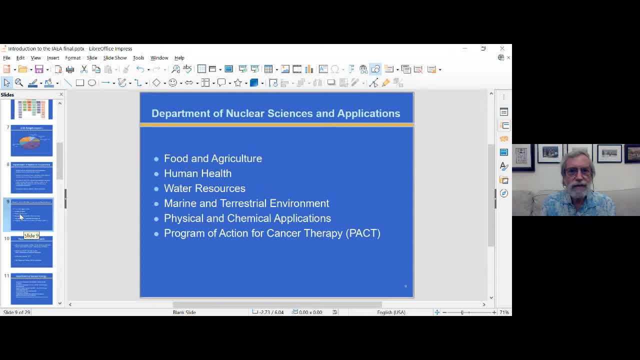 assistance related to insect sterilization, agriculture assistance, water purification, lots of things that where nuclear radioactive materials might be used in these activities and they're not obvious to a lot of us, but there are a lot of things that they can use them for that. 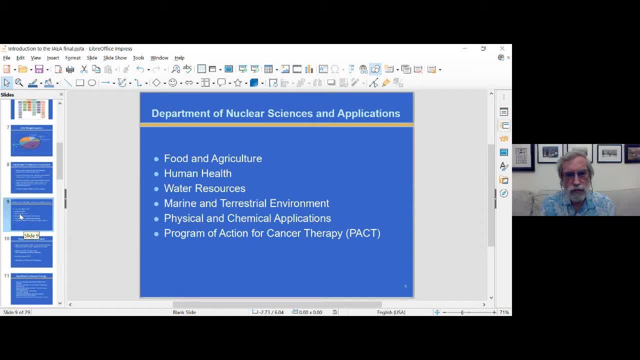 They get involved in. and again, all of these different departments would be working through the technical cooperation Department to provide these assistance. Again, all of these different departments would be working through the technical cooperation department to provide these assistance. assistance is to member states. The Department of Safeguards, As I mentioned, that was the nuclear. 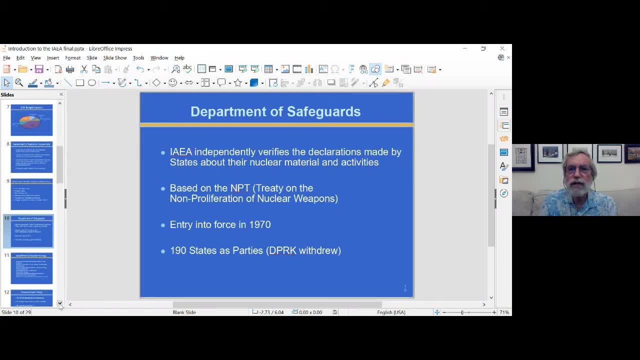 watchdogs, and what these inspectors do is they independently verify the declarations made by member states about their nuclear materials and activities, and the way they do their work is based on the treaty on the non proliferation of nuclear weapons. If you've heard about the NPT, that's what that? that's what that treaty is entered into. 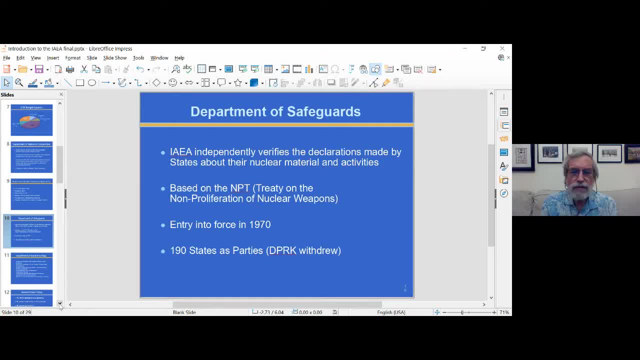 in 1970, and there are 190 states that are signed parties to that non proliferation of nuclear weapons. North Korea, which is the Democratic People's Republic of Korea. there they withdrew from the treaty a couple of years ago, so IAEA. 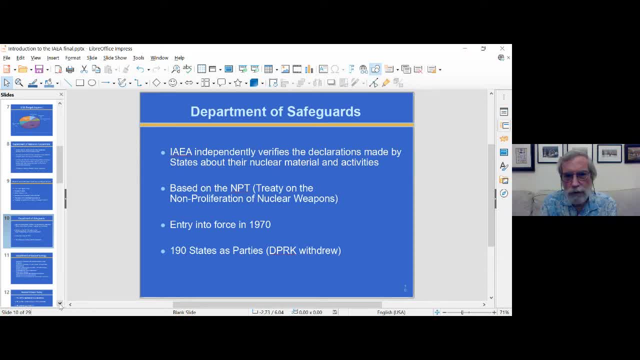 doesn't really send any inspectors to North Korea anymore, And there are some notable countries that are not signatories to the nonproliferation treaty. India and Pakistan were not members to it and have since developed nuclear weapons. Israel is also not a signatory to it, and while 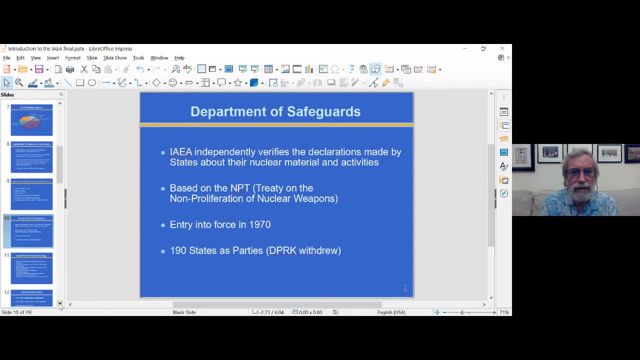 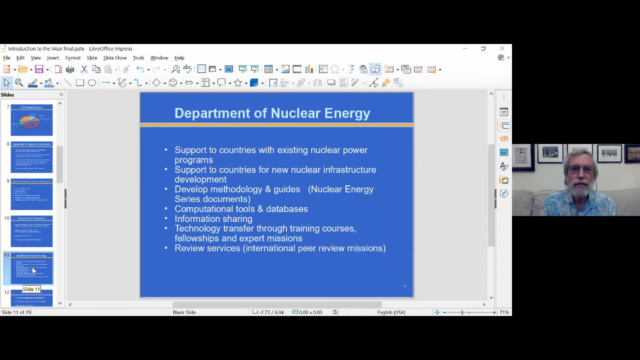 not declared. it's generally accepted that Israel might might have nuclear weapons, and so those- those countries are not- are not signatories to the treaty Department of Nuclear Energy. Again, they they provide a number of activities of support to countries with existing nuclear power programs. 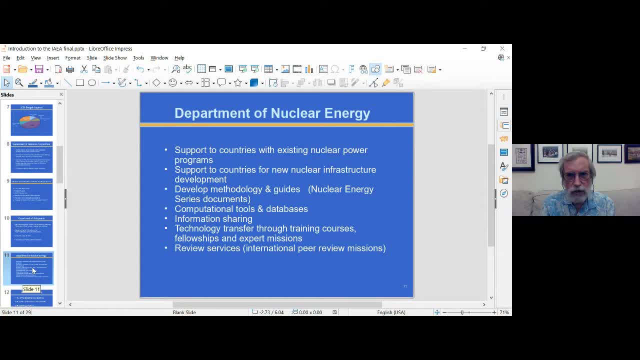 And support to countries that are either developing new programs or interested in developing nuclear power programs. And the thing is, some of the things they do. They do, in addition to providing training and guidance, they develop the methodology and guides. There's a whole series. 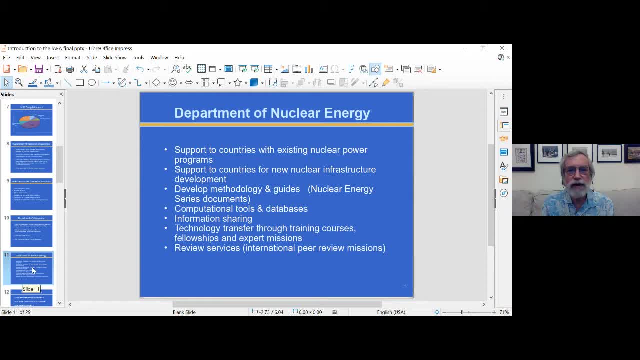 of documents called the Nuclear Energy Series- documents that provide guidance to member states on development of nuclear power programs- And you can see the other activities that they get involved in: information sharing, technology transfer and specific review services. You'll see this review services show up in a couple of different 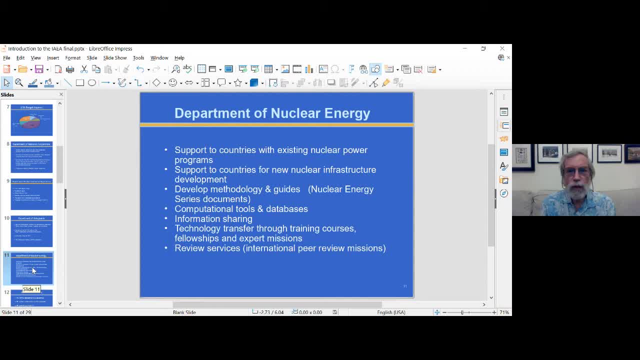 departments where, once the member states embark on their programs for either operating nuclear power plants or operating nuclear facilities or the intent to operate nuclear facilities, IAEA will provide review services where we would go in and take a look at their activities thus far. compare it. 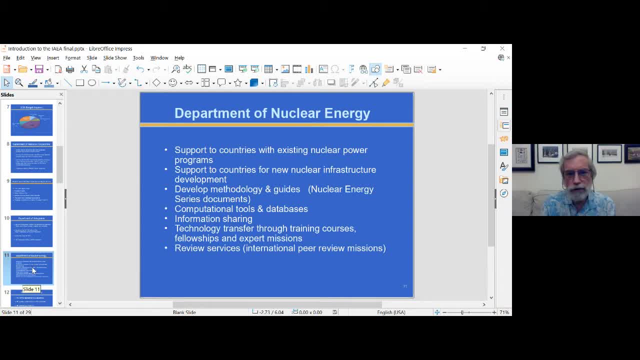 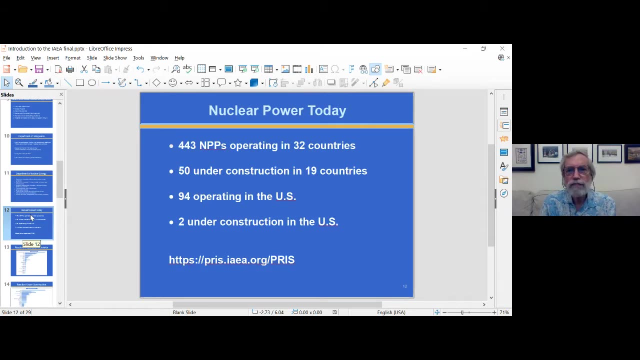 to the IAEA guidance and basically give them a report on what type of what type of progress they're making. And with regard to nuclear power, today there are 443 nuclear power plants operating in 32 countries. I took this data from the website here just just a week or two ago, so it's relatively 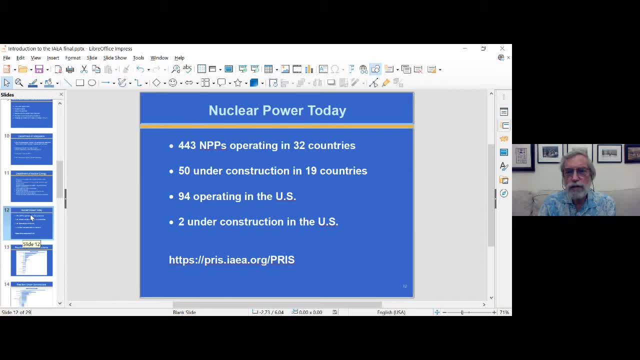 current. There are currently 50 reactors under construction in 19 different countries. Closer to home, there are 94 operating power plants in the US and two that are under currently under construction in Georgia, And this information and lots more information, is available on the IAEA website under the PRIS. 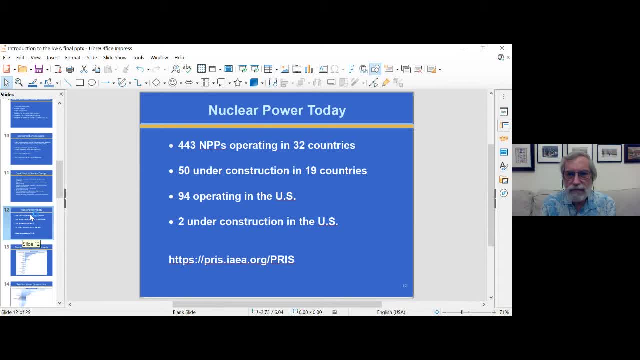 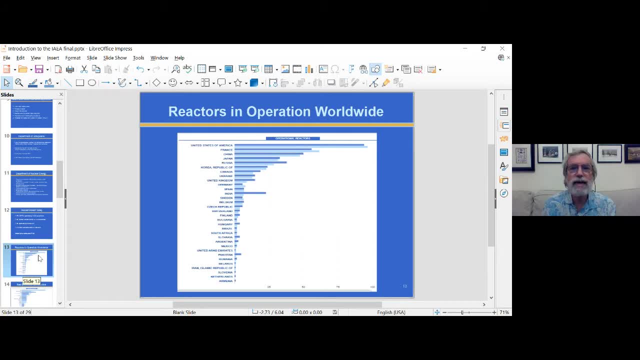 which is the Power Reactor Information System. It has a lot of detailed information about the status of nuclear power around the world. This gives you an idea of the number of reactors that are operating in these different countries, And the US right now has the largest number of power plants. followed. 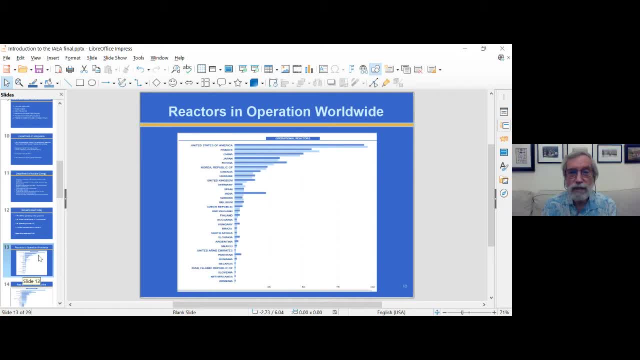 by France, China and Japan, Although it's expected within the next 10 to 15 years that China- China- may be the number one nuclear nuclear power country in the world, because they're, they're, they're building quite a few, quite a few new 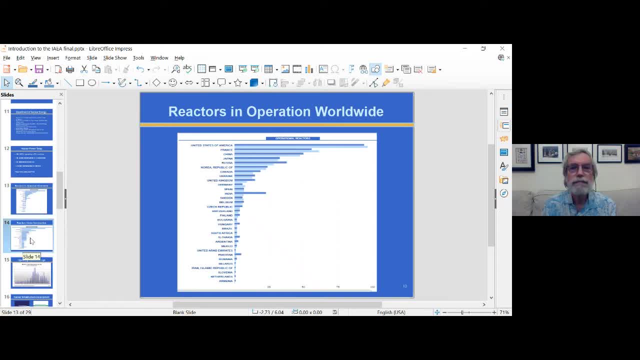 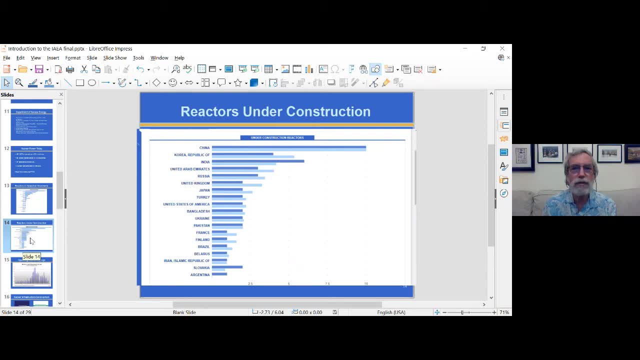 facilities right now, And the US is pretty far down the list. where we are, The US only has two, two plants under construction right now. This, this, this slide is a little bit dated. I didn't like the format of the of the current slide, but this slide is a. 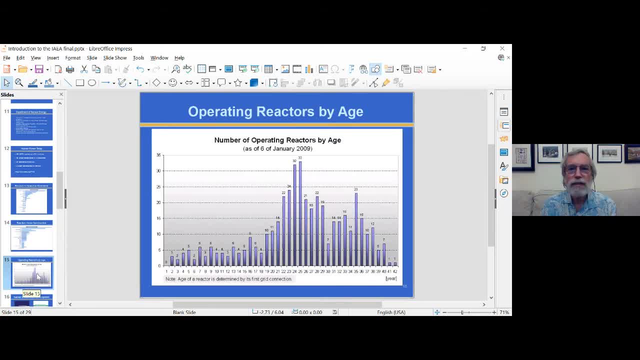 little bit dated. This, this, this slide is a little bit dated. I didn't like the format of the of the current slide, but This this is showing the age of the reactors as of January 2009,. so you could add another 10 or 12 years to this and see that the 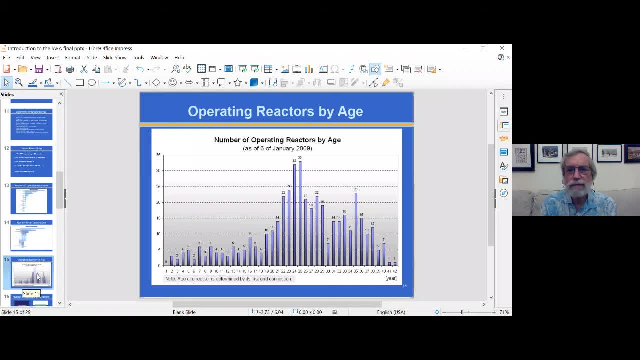 vast majority of the power plants that are in operation today across the world are, you know, there in the 30 to 35 year old range. So the nuclear fleet worldwide is is getting pretty aging And the distribution of replacement nuclear power is increasing. The distribution of replacement nuclear power is somewhat skewed. The Middle East is pretty interested in developing nuclear power. China and Russia are both building nuclear facilities. but in the West of what we consider the West Western Europe, the US, Canada are really not not building much. 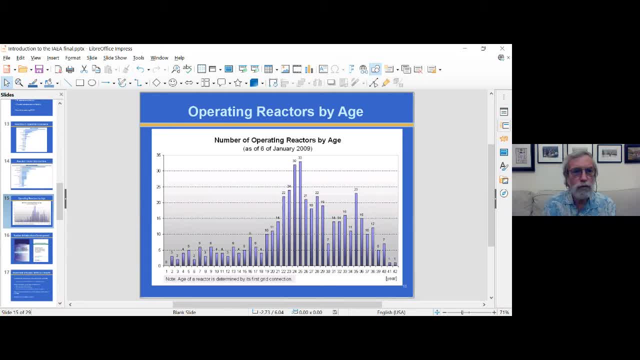 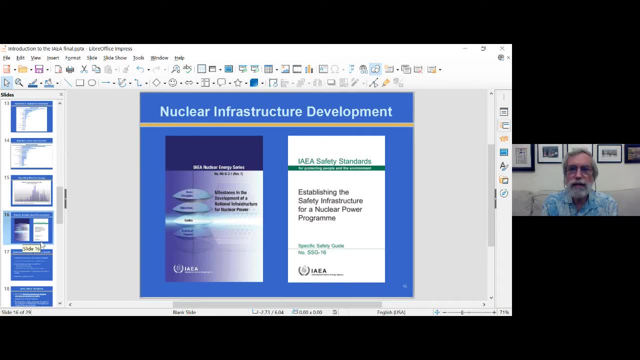 in the way of new, new nuclear power plants. This, this next slide, having to do with nuclear infrastructure development. This is for the countries that are interested in developing nuclear power. This starts forming a bridge between the Department of Nuclear Energy and the Department of Nuclear Safety. 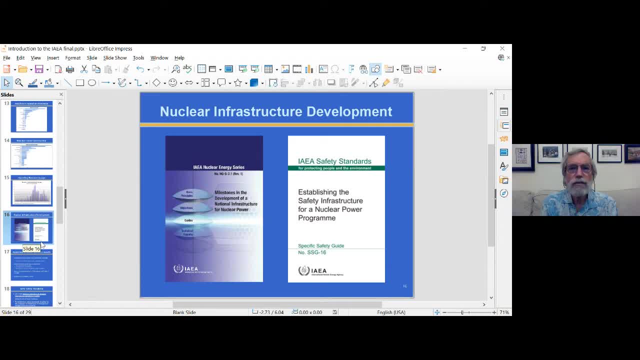 The document on the left, the IEA Nuclear Energy Series: milestones in the development of a national infrastructure for nuclear power, Provides a road map to countries that want to develop a nuclear power program and gives them Various subject areas in which they would need to develop. 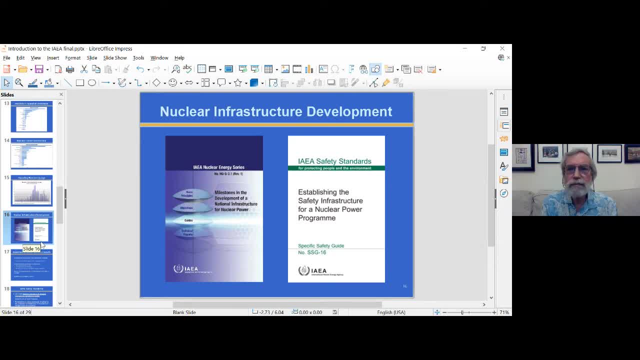 The Document on the right establishing the safety infrastructure for a nuclear power program Is a similar format in that it provides a number. it provides a listing of a number of topics that a country needs to develop A nuclear power program, but it is focusing on the safety. 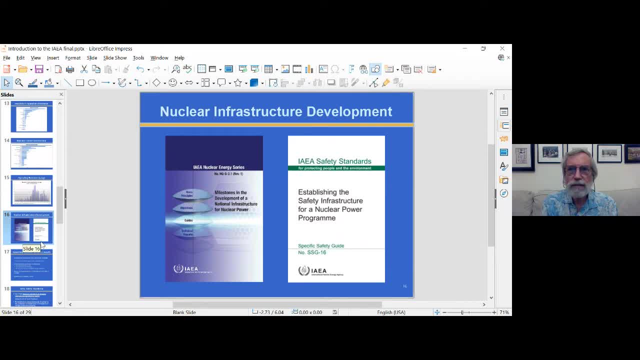 requirements associated Of With IAEA from the Department of Nuclear Safety. The nuclear energy document doesn't necessarily focus solely on the safety elements. It focuses more on the overall national infrastructure that would be required to develop a nuclear power program, taking into account many physical characteristics of the. 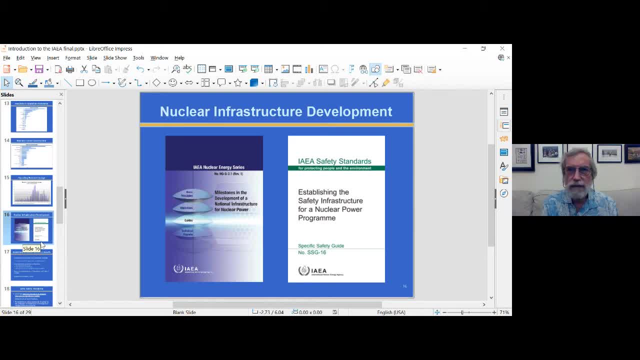 country, as well as the human resources development in a country necessary to operate, to build and operate a nuclear power program. The nuclear power program And the same things are taken into account in the safety infrastructure. that human resources development is a huge issue for countries that want to develop nuclear power. 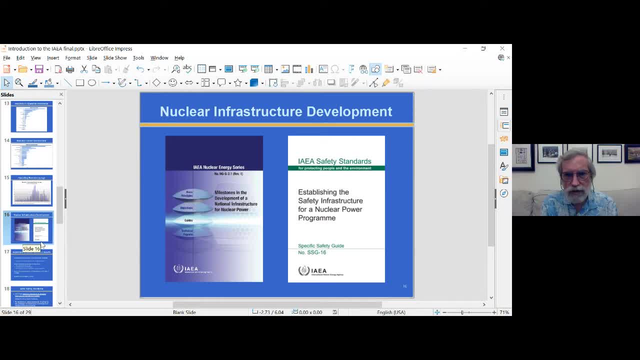 A lot of times people focus on nuclear engineers and nuclear physicists with regard to human resources development, but the development of a nuclear power program takes a huge array of Of engineers to develop. it needs the country. The country needs to have a good program for developing mechanical engineers. 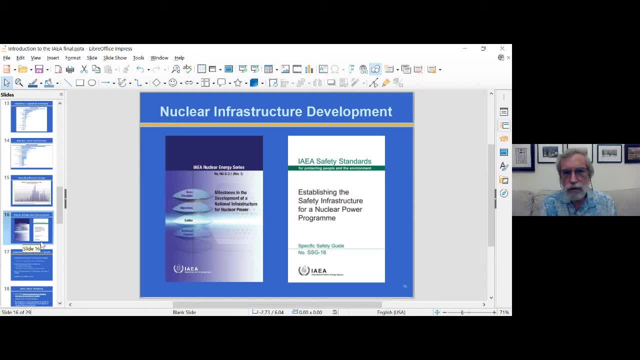 electrical engineers, civil engineers, chemical engineers, structural engineers, Hydraulic engineers, just any, any number of Disciplines are necessary to for a functioning nuclear power program. While you do need a certain core of nuclear physicist and nuclear engineers, those other types of engineers can get them, can get the nuclear training. 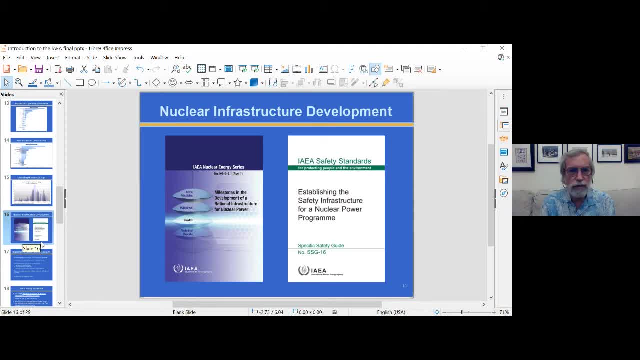 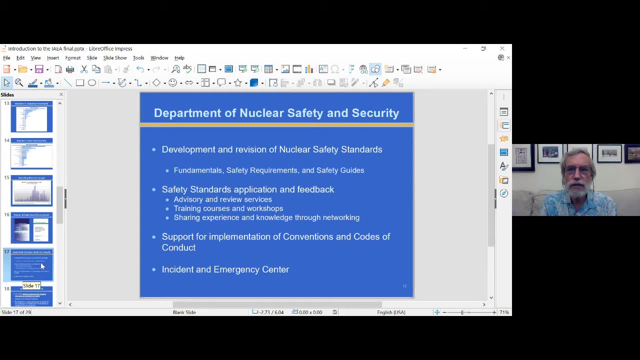 And then you can get the nuclear power program And it's really important that you have a well rounded human resources development program to be able to develop and support a nuclear power program. Getting more specifically to the Department of Nuclear Safety and Security, I made that bridge from nuclear energy to nuclear safety and security. 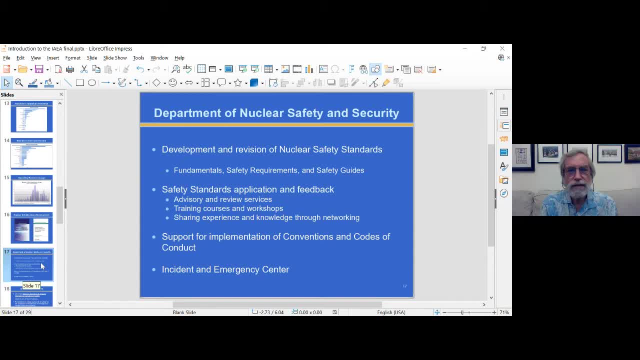 The functions that this department did, which was the department I was in. we were responsible for the development, The revision of nuclear safety standards, which includes fundamental safety requirements, safety guides, the application of the safety standards and feedback to member states, Support for implementation of conventions and codes of conduct, and IAEA also operates. 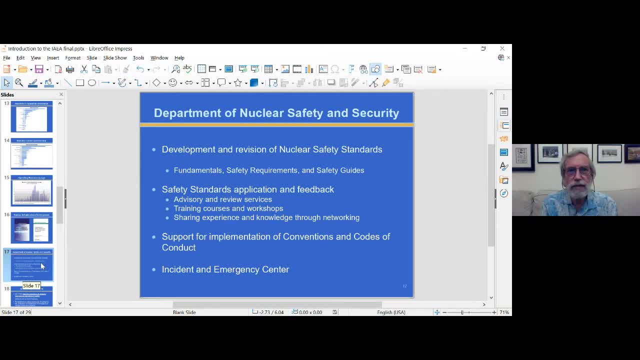 an incident and emergency center in there in the Vienna International Center. there in their headquarters in Vienna. the incident emergency centers are pretty important Center there. It coordinates information regarding radiological and nuclear incidents worldwide. It was probably the last major incident that we got involved in. 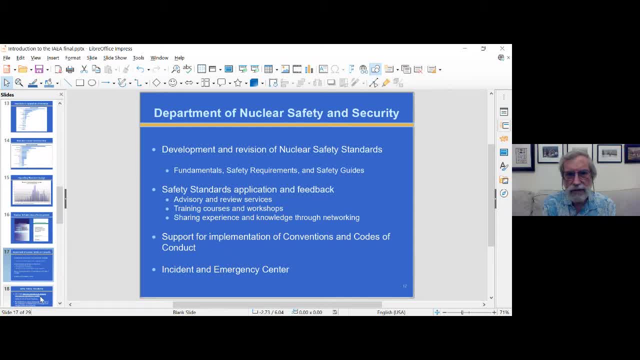 There was the Fukushima accident back in 2011.. I was a pretty active participant during that, during that event, and that went on for weeks and months. So the incident response center was staffed 24 hours a day and while there's a core staff for the incident emergency center, 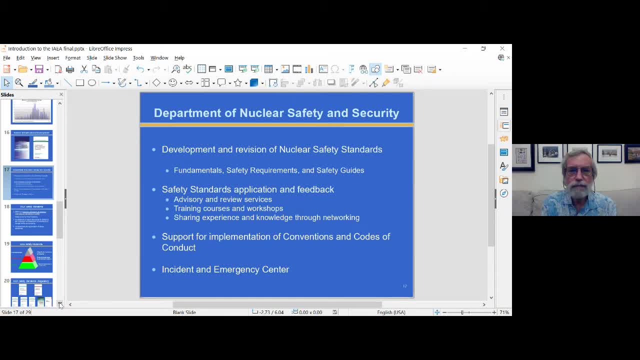 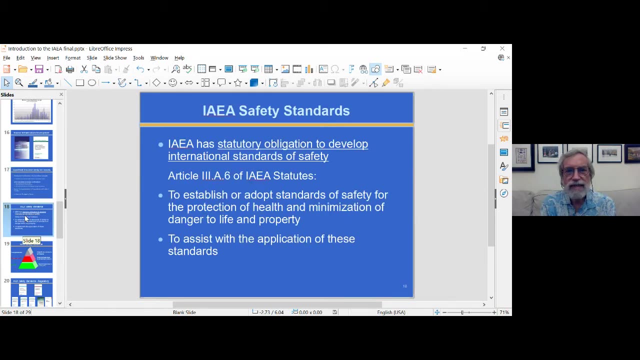 it draws on the other technical departments in IAEA for staffing to make sure that it can, that it can run and function as long as necessary. The IAEA safety standards again is one of the main tenants of the Department of Nuclear Safety and Security. 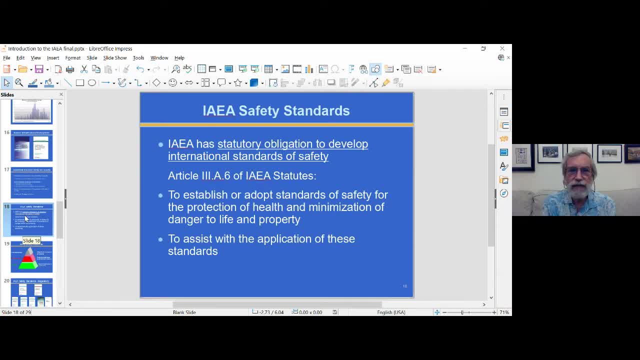 We were responsible for developing the international standards for safety as part of the IAEA statute, And what those are for is the protection of health and minimization of danger to life and property, and we assist member- We assisted member states with the applications of those standards. 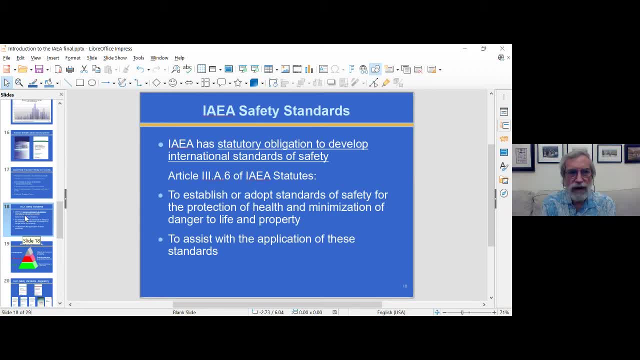 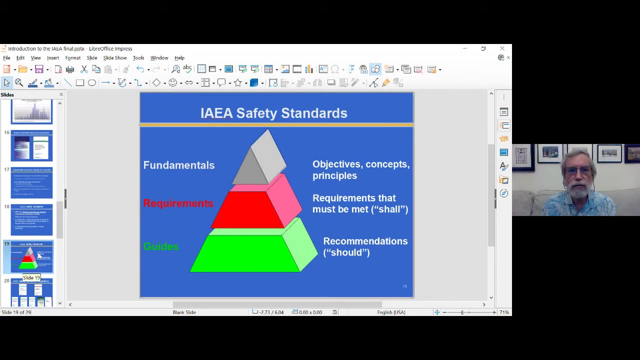 In addition to developing the standards, we also provided guidance for the implementation of those standards and the review of the implementation of those standards through the various review services. The safety standards has three different levels: fundamentals, requirements and guides. You can see there what what they cover: the objectives, concepts, principles, requirements. 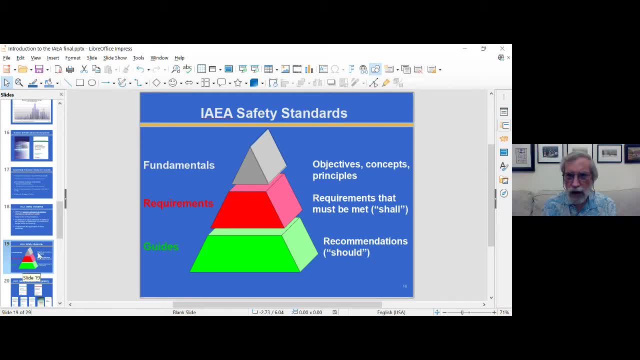 These are things that they're required to do, and then guides are things that they should do, And these things are implemented via conventions. I made mention earlier of some conventions. there. There are a number of conventions. There are a number of conventions that IAEA oversees, and one of them is the Convention. 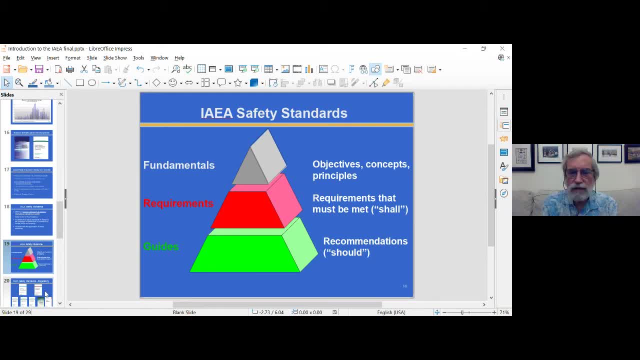 on Nuclear Safety. Member states sign up to these conventions, which they are agreeing that they will abide by and implement the safety standards of the IAEA in their nuclear and radiological activities. And this is just a- if you want to call it a- quick rundown of a particular safety standard. 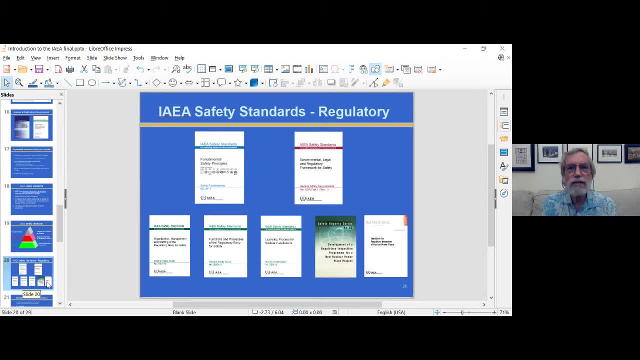 And this is just a- if you want to call it a quick rundown of a particular safety standard. This is just a- if you want to call it a quick rundown of a particular safety standard. There is a competitors set of safety standards for the regulatory field. 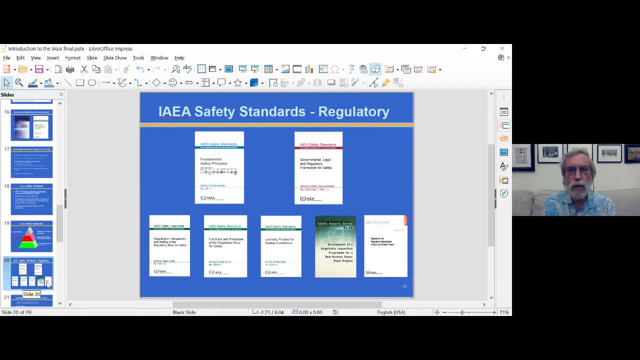 If you have this fundamental safety principles, which applies across the board to all aspects, Then there's a more specific safety requirement, that's, governmental, legal and regulatory framework for safety. This will provide guidance to member states on what they need to do to develop a 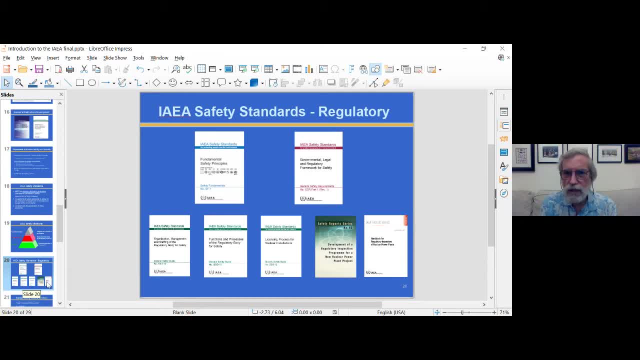 legal and regulatory framework for safety. example of that in the US would be: the Atomic Energy Act of 1954 is the legislative act that provides for a nuclear power program and oversight program in the US- The Atomic Energy Act of 1954. 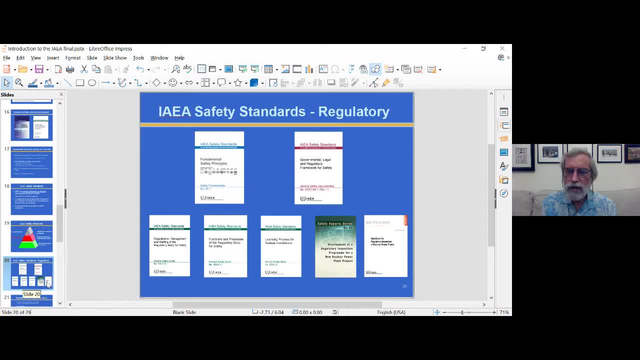 established the Atomic Energy Commission, and that went on for a number of years. What turned out to be, I want to say, a problem, but an issue with the Atomic Energy Act, was it provided the promotion and regulation of nuclear power under the same legislative and 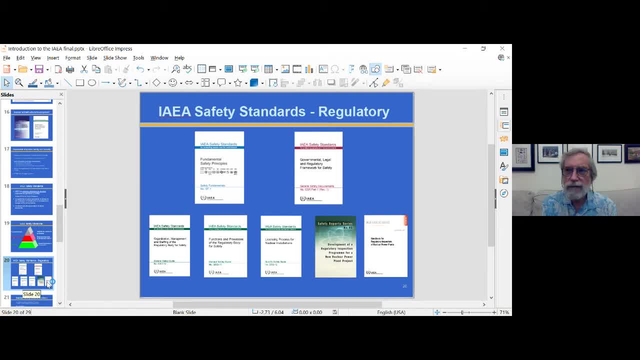 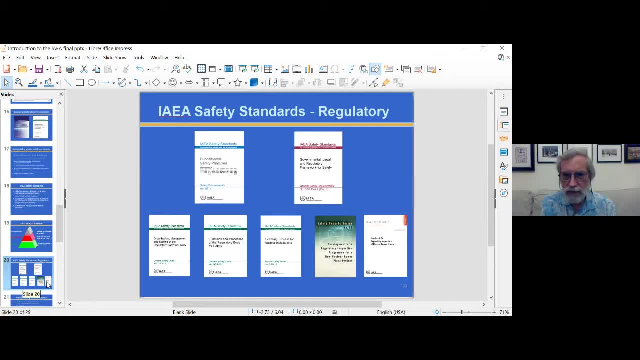 talking about- And that's what we're talking about, And that's what we're talking about- The NRART Failure Regulatory Commission from what later became the Department of Energy. So now the Nuclear Regulatory Commission's sole function is regulation. It's not involved in promotion. and the Department of 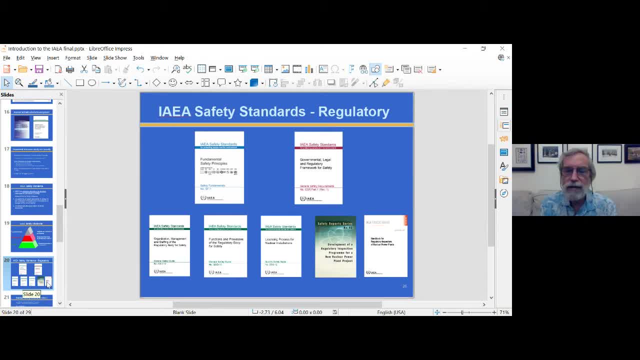 Energy is now responsible for promotion of nuclear activities on a national level And then underneath the Safety standards. there are a number of safety guides. These are just a couple of examples of safety guides: Organization of the regulatory body, functions of the regulatory body, licensing process for nuclear installations. 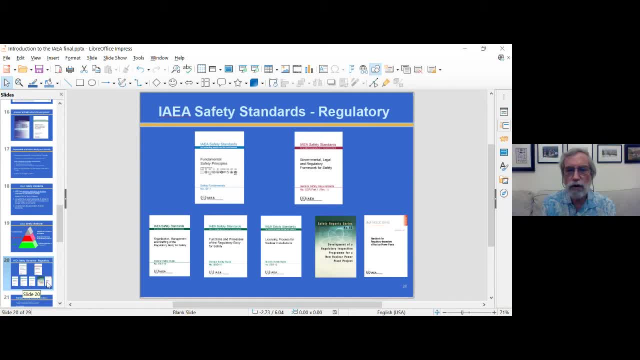 Those are all activities that a regulatory body would normally perform, And this provides some guidance for regulatory bodies to perform those functions. Again, this is just a sample. There are a number of them And there are safety requirements and safety guides covering many. 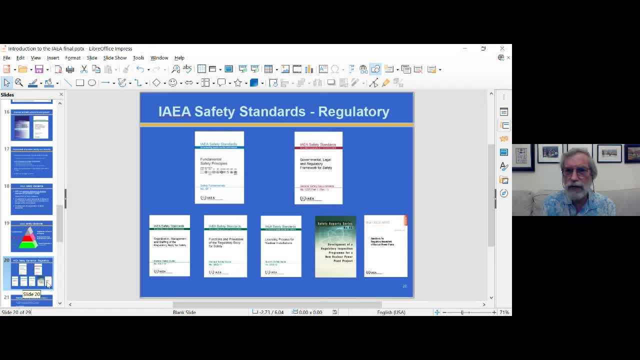 many different areas. This just happens to be one for the regulatory body And in addition to the safety guides, there are lower tier documents, the safety report series and technical documents, ie a technical document. They provide information, more information regarding. 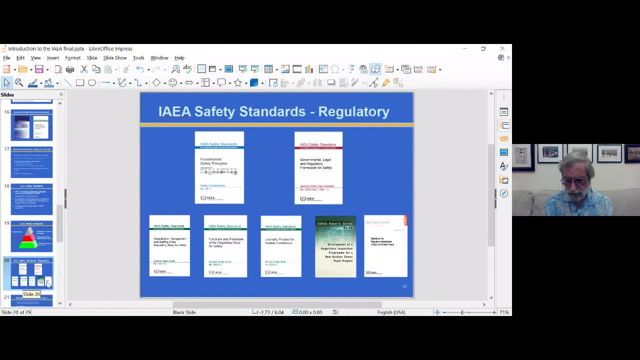 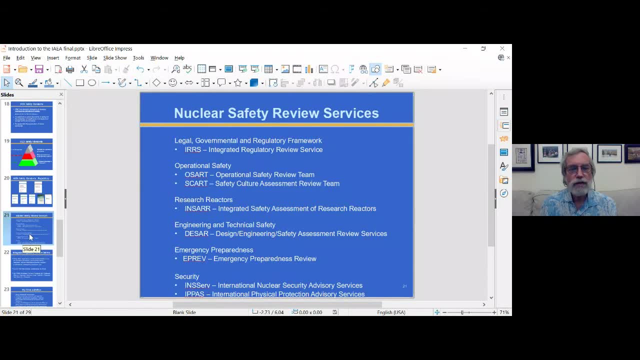 various topics, but they don't rise to the level of even a safety guide. Again, as I mentioned earlier that I'd be focusing more on what functions I did and our organization did In the Department of Nuclear Safety, there are a number of review services. 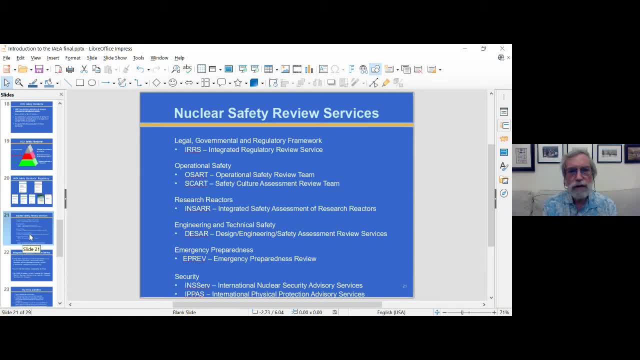 that are conducted, And these review services are organized and coordinated by IAEA And they go out and verify the implementation of safety standards. in these various subject areas- The legal, governmental and regulatory framework- we had a mission called the Integrated Regulatory Review Service Mission, which was one that I was very heavily involved in. 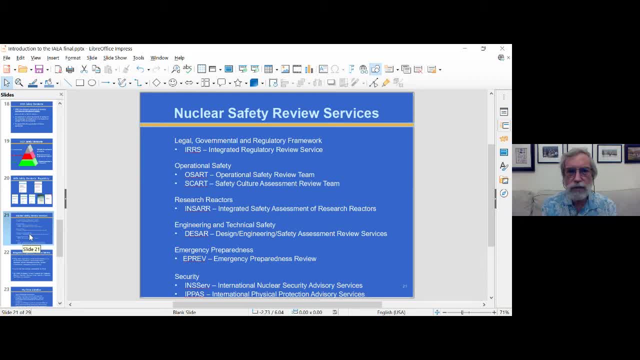 From an operational safety standpoint, there are a couple of review missions. There are also missions for research, reactors, engineering and technical safety, emergency preparedness, security. So all of these different subject areas have safety requirements associated with them and associated review services to see how member states are in fact implementing those. 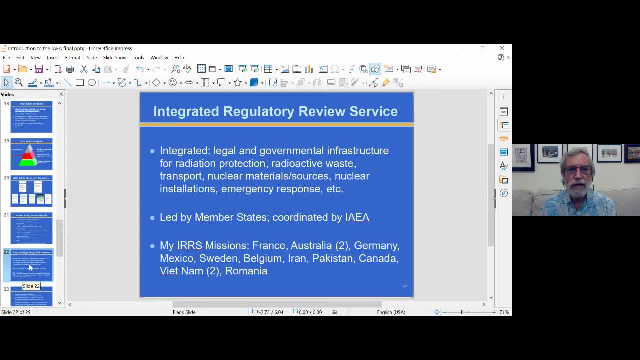 The Integrated Regulatory Review Service, the IRS mission. that was a. it's called integrated because it takes into account not only the nuclear power side of the house but also radiation protection, radioactive waste, radioactive transport of materials, nuclear materials and sources, nuclear installations- emergency response. 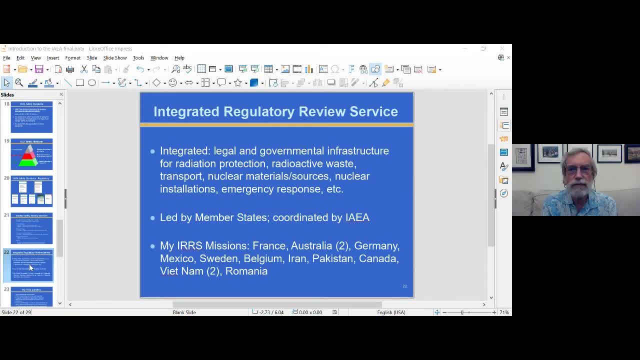 All of those different activities were folded into the Integrated Regulatory Review Service. The teams are led by member states but coordinated by IAEA. My function would have been to put the team together. A member state would come to us and request a review mission. 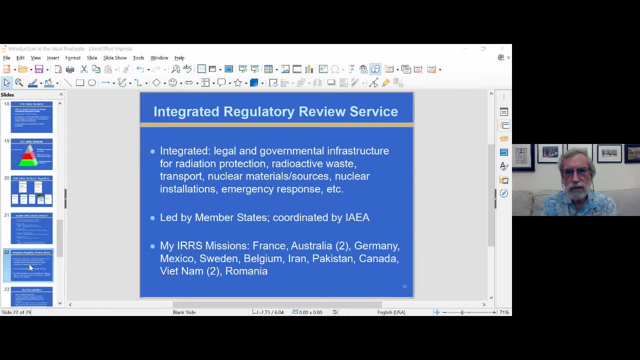 So I'd be involved in that and the team would be part of that. So I'd be involved in that and the team would be part of that and the team would be part of that. None of these review missions are mandated by IAEA. 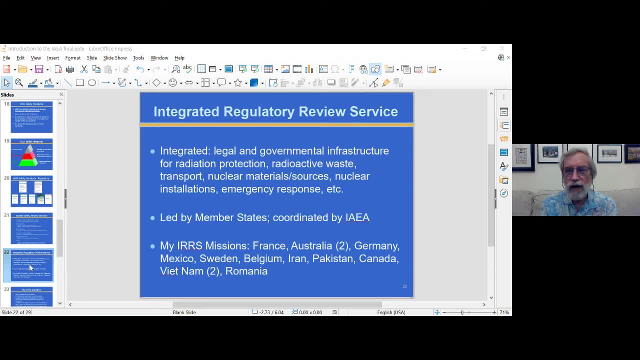 They are strongly suggested and recommended, but they're voluntary by the member state. They have to request it. Once they request it, a coordinator would be assigned and the coordinator would start assembling a team and determining the scope of the mission, And the team itself would be led by representatives from member states and the team members would. 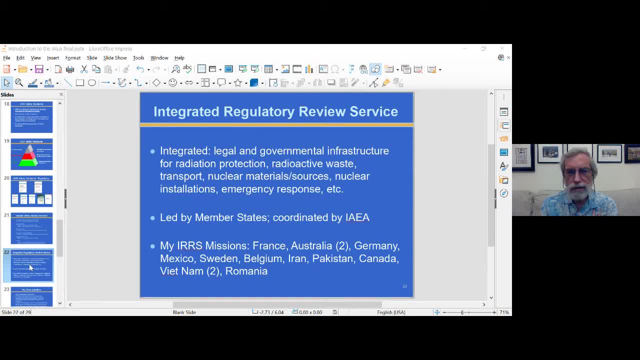 all come from member states. For a full-scope mission, a team would typically be 20 to 25 persons, and the review mission itself would typically last two weeks, but the preparatory work for that mission would start probably about a year early. 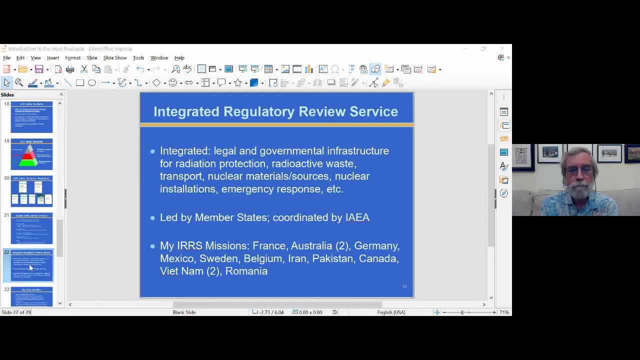 It would take nine months to a year to put the mission together, conduct the mission over a couple of weeks and the report would be issued officially within three months or so after the end of the mission. The missions that I was assigned, The missions that I was directly involved in, were the ones listed there: France two. 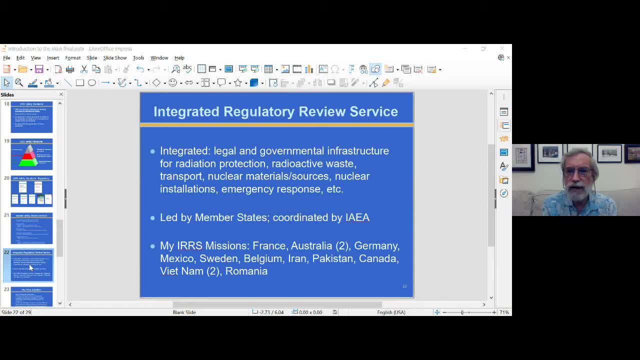 in Australia, Germany, Mexico, Sweden, Belgium, Iran, Pakistan, Canada, two in Vietnam, Romania and also in Vietnam. Not only did we do the safety review service mission, but we also did the nuclear infrastructure review from the nuclear energy standpoint. 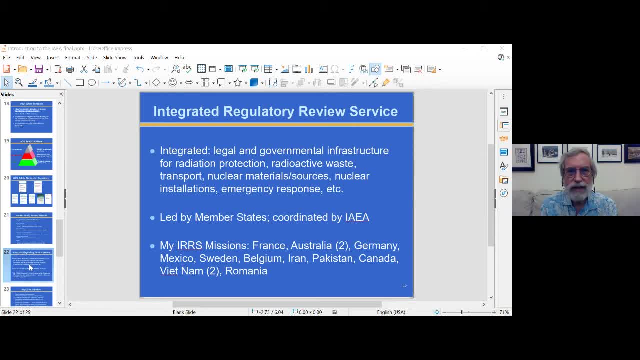 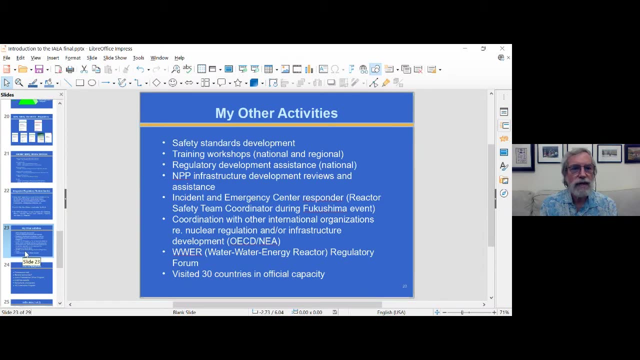 Which takes a slightly different approach, Completely different scope, and interacts with different people, but is looking at some of the same subject areas. Other activities that I got involved in directly, in addition to the IRS missions, were the development of safety standards. We conducted training workshops, both national and regional, typically through the technical 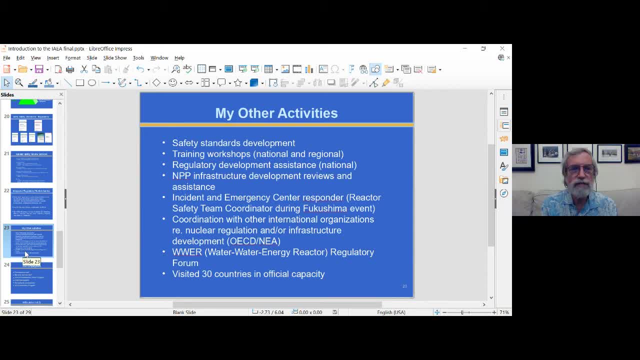 cooperation program where member states would request various training missions On certain topics and we would put together workshops to address those needs. Same way with regulatory development assistance, In addition to just training workshops. they may also ask us to review certain documents of theirs or certain activities that they have ongoing, and we would provide them some. 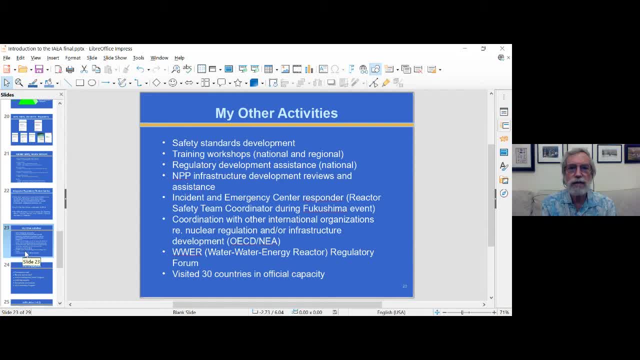 feedback on those activities. We also conducted the nuclear power plant infrastructure development reviews and assistance, As I mentioned earlier. the incident and emergency center responder. We also conducted the nuclear power plant infrastructure development reviews and assistance, As I mentioned earlier. the incident and emergency center responder. 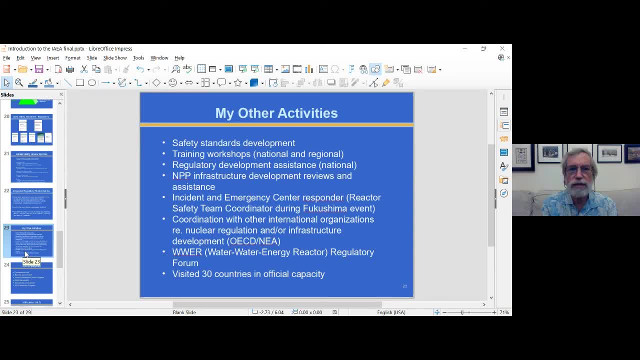 During that Fukushima event I was the reactor safety team coordinator. during my shifts when I was up there, I usually had two or three reactor safety specialists working with me to perform those functions. We also coordinated with other international organizations, specifically with us for nuclear. 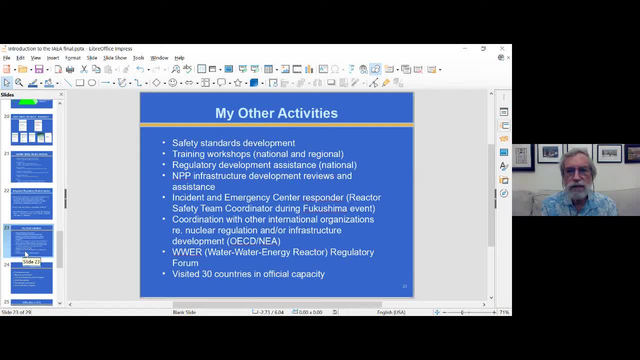 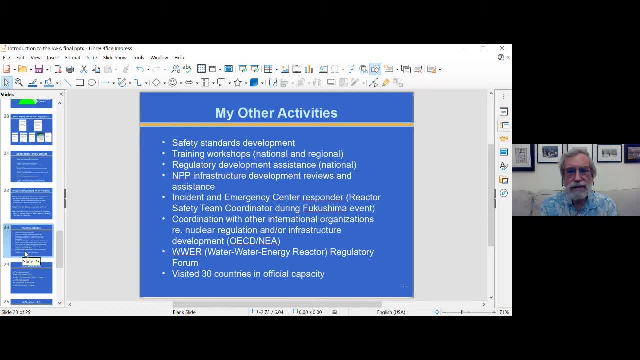 There are other than the first two. There is a special regulatory forum, that is a water energy reactor regulatory forum, The water water energy reactors. as a is a Russian design pressurized water reactor. that there's a regulatory forum where operators of those particular reactors would meet. and 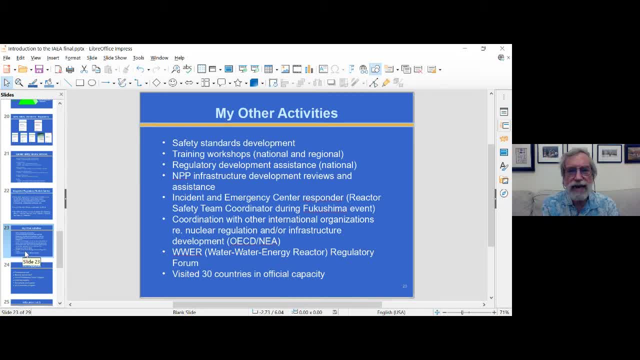 discuss technical issues and Interact with alpha, And we would interact on what I was doing with regard to regulatory activities and so on. And during my time at IE, I visited over 30- over 30 countries and in my official visits I did. 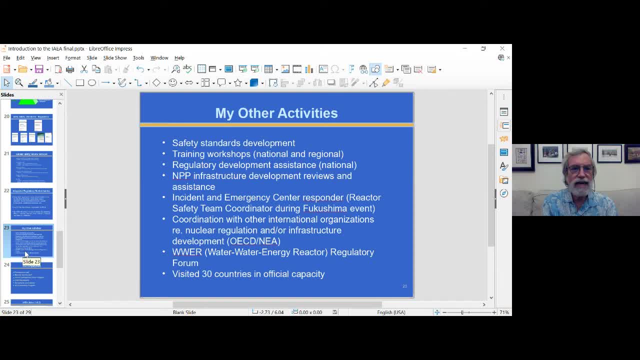 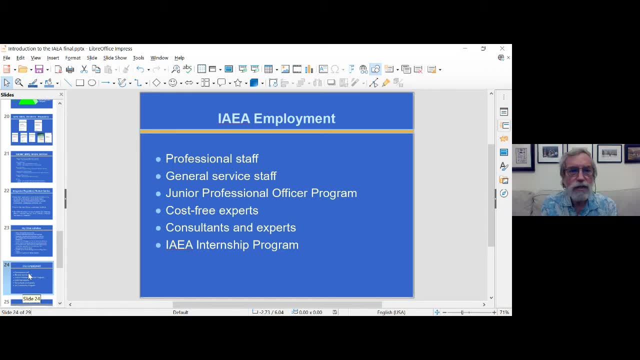 I had more than 2,030 visitors in my official visits, So I had more than 2,030 visitors, So we had more than 2,030 visitors capacity. So then, a question may come up about about working for IAEA: The. 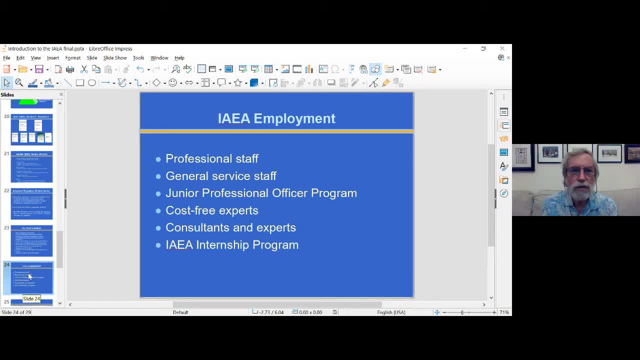 various the various jobs, about how you get into IAEA and what they do. The professional staff is typically very experienced. They don't the. the normal path is is for most of the staff is they don't want IAEA doesn't want to train people technically. They want people that are already trained with lots of 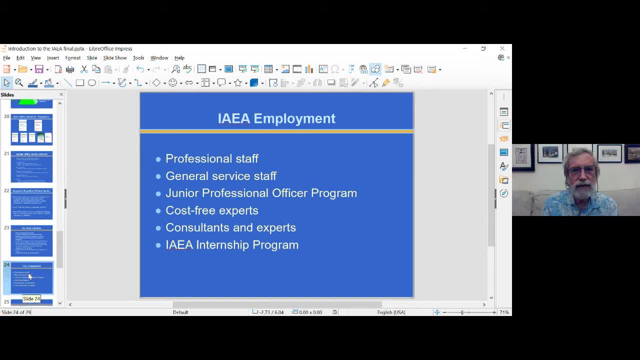 experience and to bring them in at a fairly high professional level, and then you just have to to learn the IAEA bureaucracy and administrative processes. General services staff is typically the admin and clerical staff. They also have a junior professional program, junior professional officer program, which is 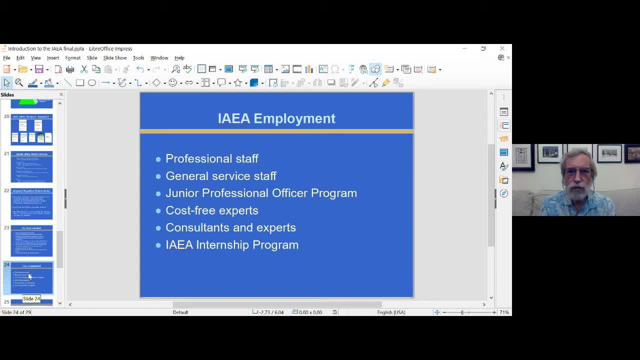 where they take typically people right out of school, and they will. they will come in as a junior professional and one in some one of the departments, and it's typically a one-to-one two-year program where you will participate in the activities for whatever department you're in and basically start developing your 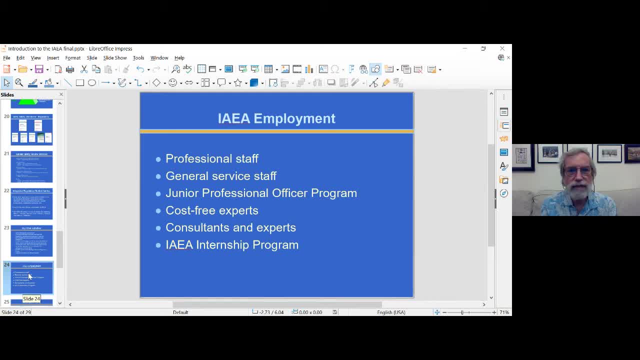 professional expertise in some field related to IAEA activities. Cost-free experts are typically experts from member states, where they are supplied to IAEA and the member state pays for them to to work at IAEA. Then you have consultants and experts who typically work on short-term. 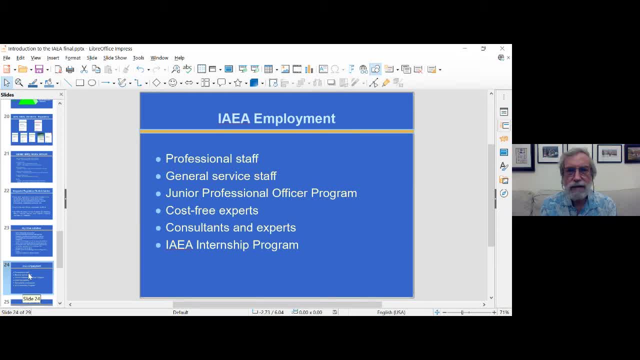 short-term contracts or specific activities or tasks for IAEA. and then there's also an IAEA intern internship program where they'll bring in interns that are not even technically part of the professional staff but they get involved in various activities related to IAEA and they typically last can last. 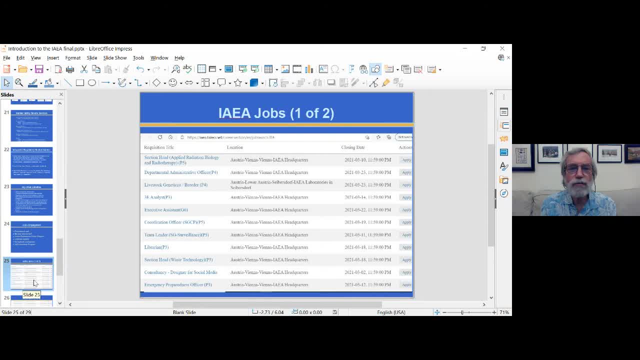 up to a year. This was a couple of slides that just shows what types of jobs are available at IAEA now. I took these screenshots just from a couple of weeks ago, so the vast majority of positions are in Vienna and they run the range all the way from. 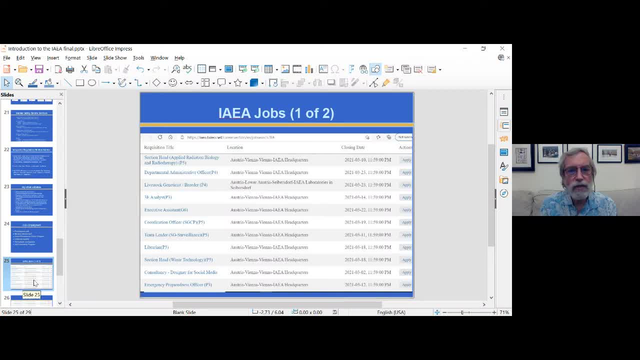 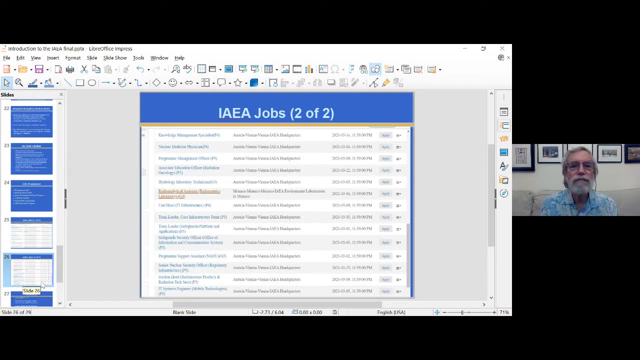 admin type staff. you know librarians, they have consultants, emergency preparedness staff, livestock geneticist and breeder, IT staff. you know just any number of any number of activities: Radiation officer, knowledge management, specialist nuclear medicine, again the senior nuclear security officer. it. 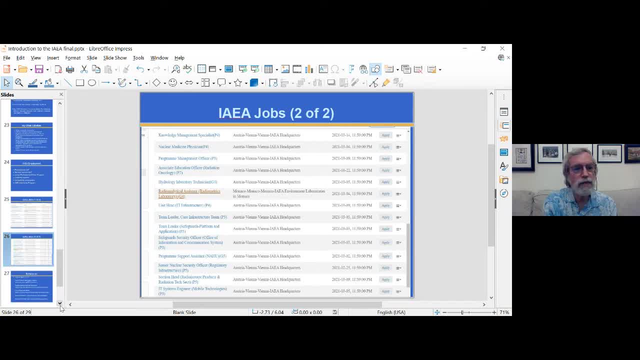 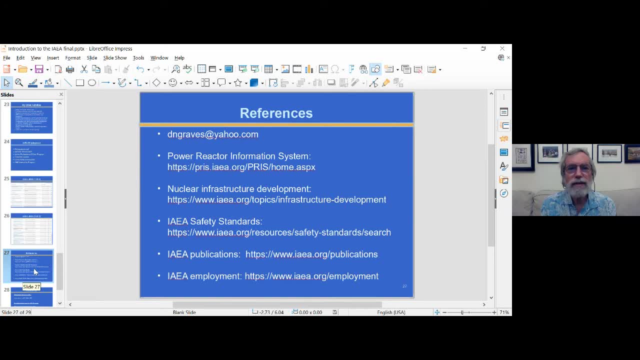 covers a wide, wide range of professional disciplines. I also had a provide a list of references here. if somebody wanted to ask me a specific question later, they're welcome to speak in the chat. And then there's my email address. There's the website address for the. 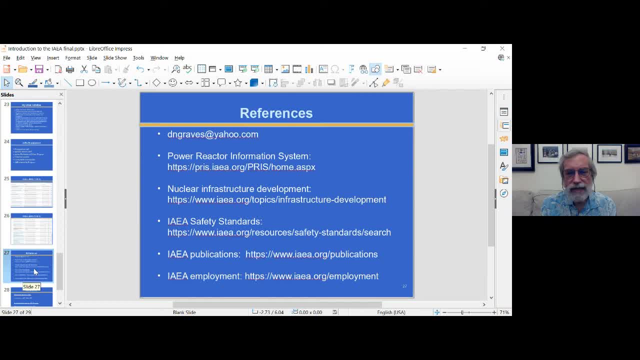 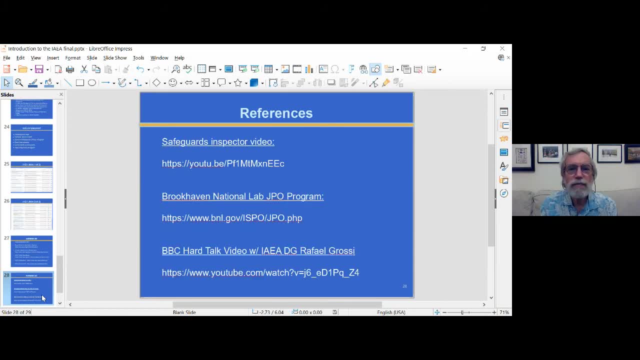 power reactor information system. nuclear infrastructure development, IAEA safety standards. various other publications, IAEA employment. a couple of other videos on here: the safeguards inspector. safeguards inspector video. This particular individual is a graduate of a University in Texas, came into IAEA under that junior professional officer program and was involved in that program. 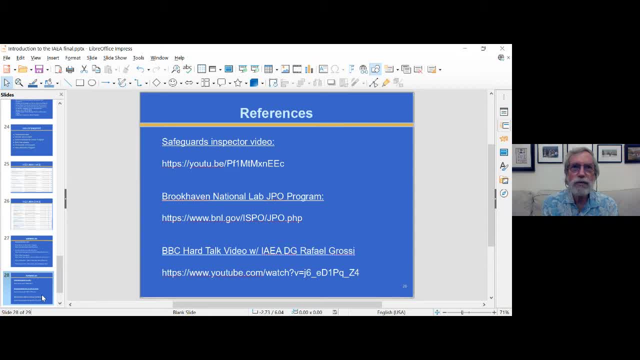 for a year or two And then eventually eventually ended up becoming a safeguards inspector, And this is a short video about five minutes that gives you a brief overview of her job, what she does when she goes out on an inspection and what a safeguards inspector does. And in addition to this, 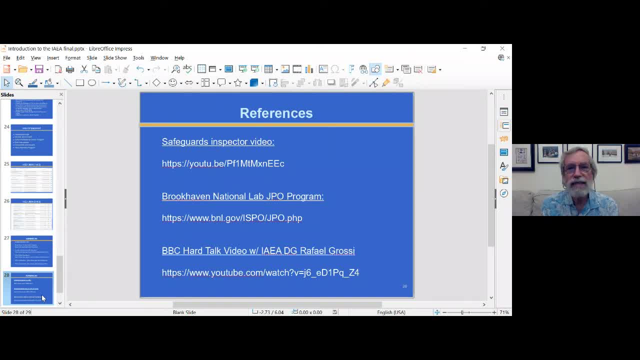 video. while it's interesting, there are many videos on the IAEA website that describes what different activities the IAEA is involved in and describes a lot of different jobs and review services and things like that Gives you a lot of information. The junior professional. 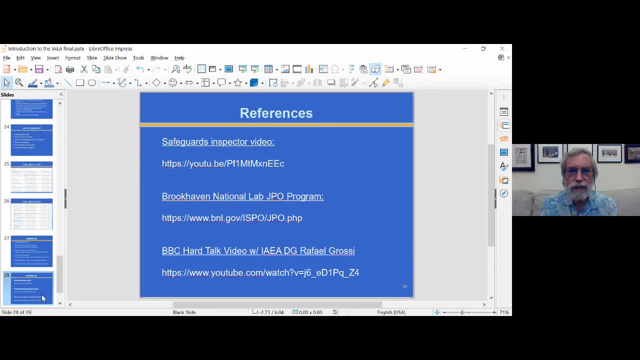 officer program is run by Brookhaven National Laboratory And this is the website for that program for anyone that may be interested. There was also an interesting BBC video. They have a program called Hard Talk And there was an interview with the new IAEA DG, Rafael Grossi, from Argentina. It was just a few weeks ago And 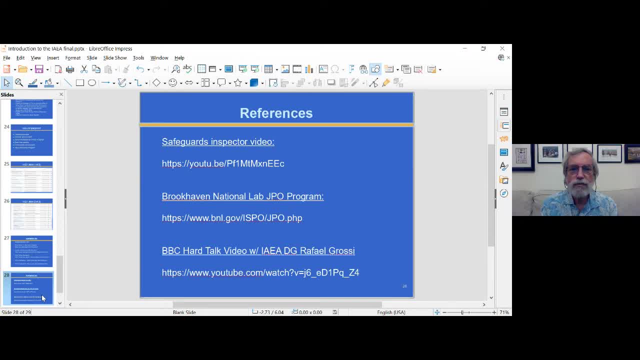 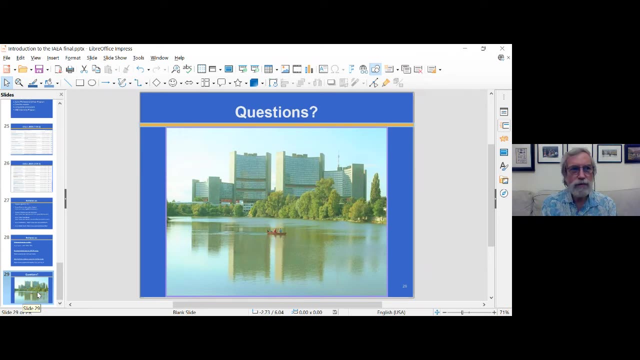 that was a pretty interesting video, So I thought I'd put the address for that talk on there. I found it pretty interesting. So with that, that's the end of the information that I had intended to provide. I know I went through it pretty quickly, But again, just in summary. the IAEA provides support. 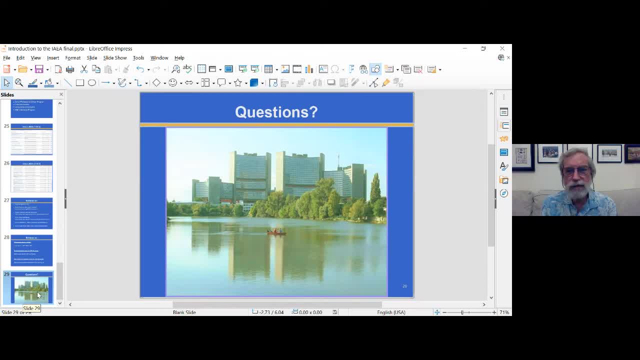 to member states in a really, really wide range of nuclear and activities, for nuclear activities and radiological aspects, both from a source standpoint and a nuclear professional standpoint. This photograph shows the Vienna International Center and the National Center, So I think it's a good example of kind of from a distance, But that whole. 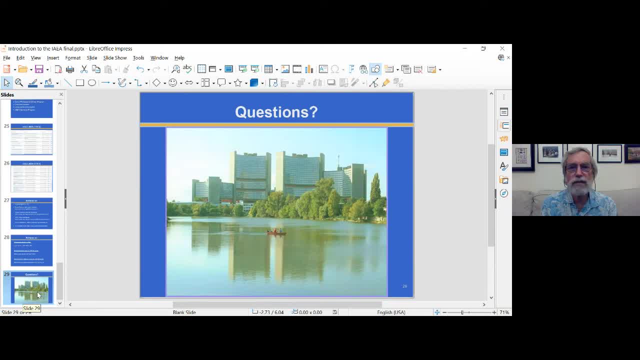 complex there. not all of it is IAEA. There are a number of UN organizations that are housed in that Vienna International Center. The biggest one is IAEA, But there's also a illicit drug trafficking organization there. There's what's called CBTBO, which is the Comprehensive Test Ban Treaty. 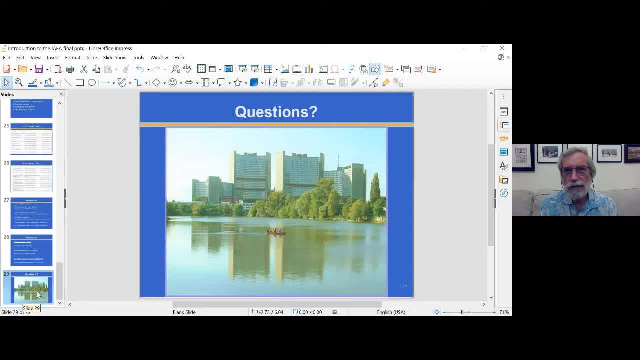 Organization, which is the organization that monitors the globe for nuclear weapons. So that's kind of the big one, And the other one is the National Center for Nuclear Abuse. All right, Thank you, Thanks, Thanks, Thanks, Thanks Thanks. 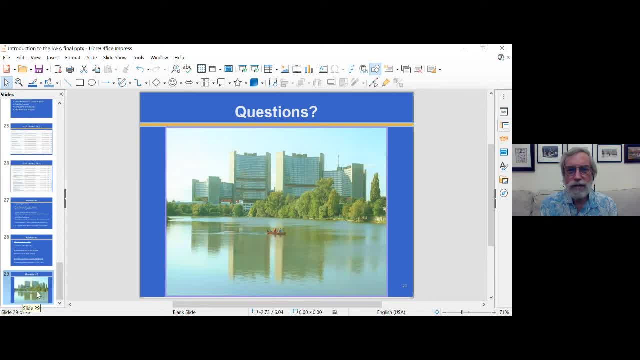 testing, which is an interesting organization, and their headquarters is in Vienna. Also an organization called UNIDO, which is the United Nations Industrial Development Organization. their headquarters is also in Vienna. So with that, I guess I'll pretty much end the presentation and see if anyone has any questions. All right, thanks a lot, David. 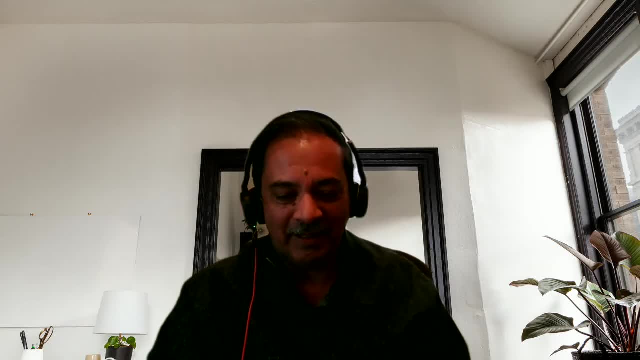 And this was really excellent and wonderful presentation and it was very informative. And I for sure did not know that IAEA is involved in so many nuclear related activities, So I don't know how we do a virtual applause. I'm not sure, but from all of us a big thank you. 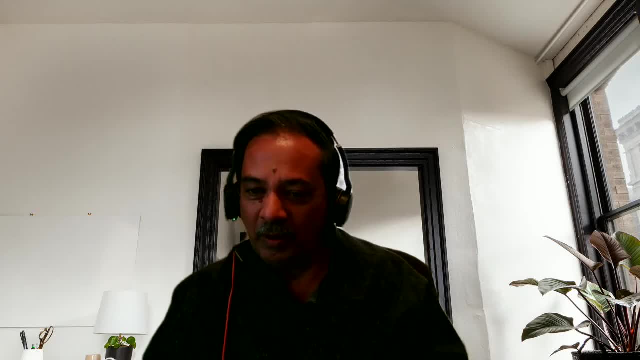 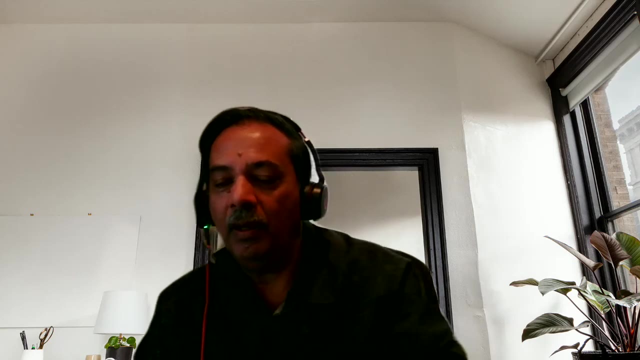 for that And I'm going to now talk about. let's see if we have any questions. Yeah, we have two and it seems it's coming from the same individual. So the very first one kind of interesting, relevant to the current situation. 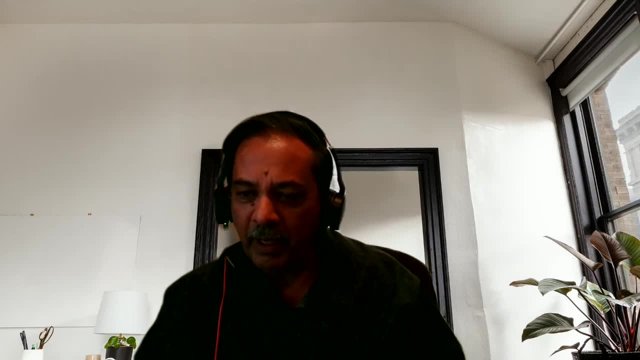 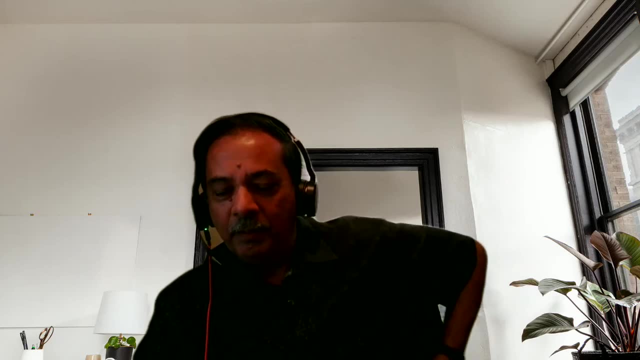 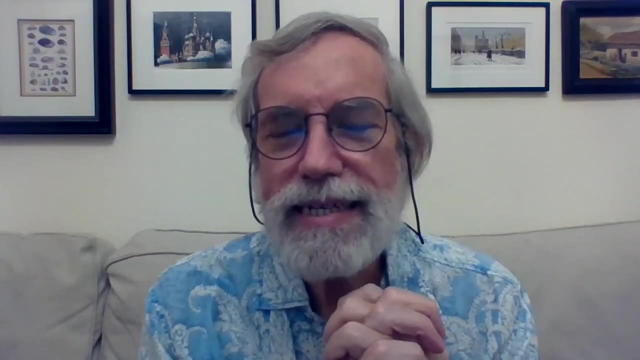 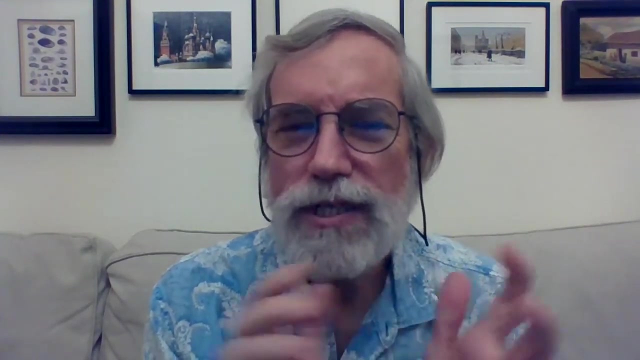 And he's asking that: how is the current pandemic with regards to SARS and COVID affecting the operation of IAEA? Yes, from my friends and colleagues that are still working at IAEA, the vast majority of them are working from home. Many of their activities are, I don't want to say. 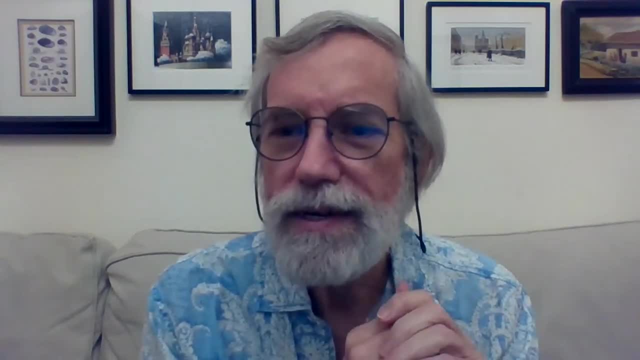 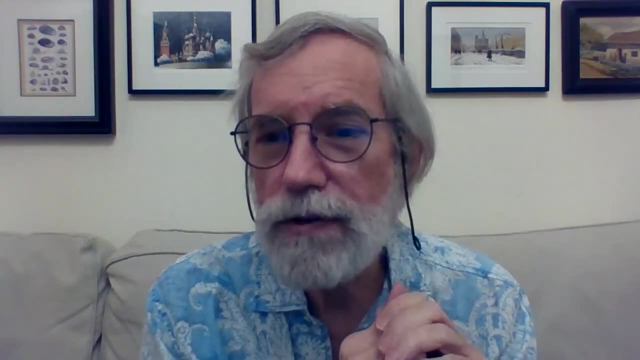 administrative, but you know they're technical paperwork in nature- scheduling and coordinating- So a lot of that can be done remotely. The inspectors that actually go out into the field- some of them, they're still doing their jobs- They're going out into the field and 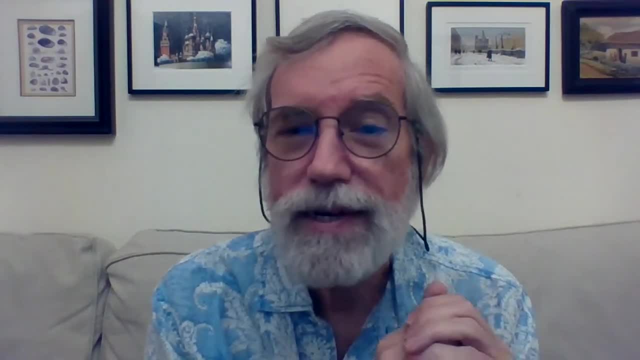 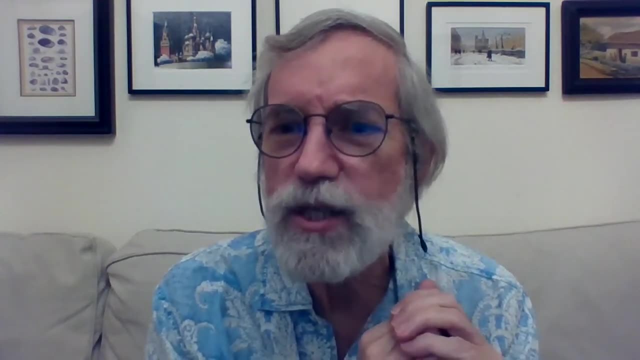 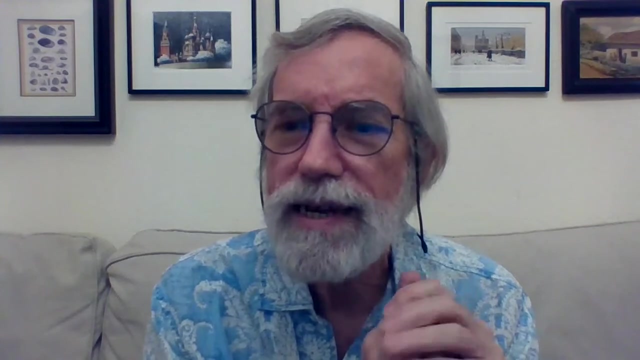 conducting safeguards inspections, as they have to. But some of the staff is still coming into work, but they're doing it on a case-by-case basis. They reviewed- apparently reviewed- all the different jobs there at IAEA, saw which ones could be done remotely. 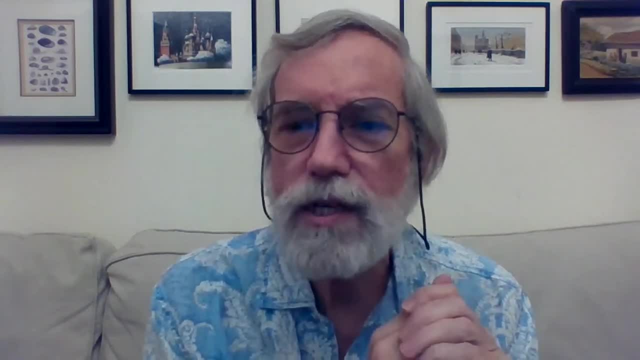 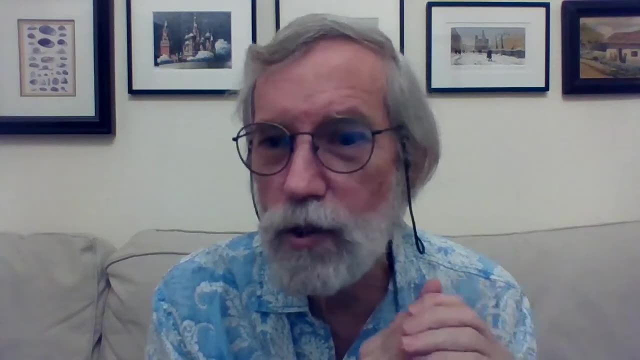 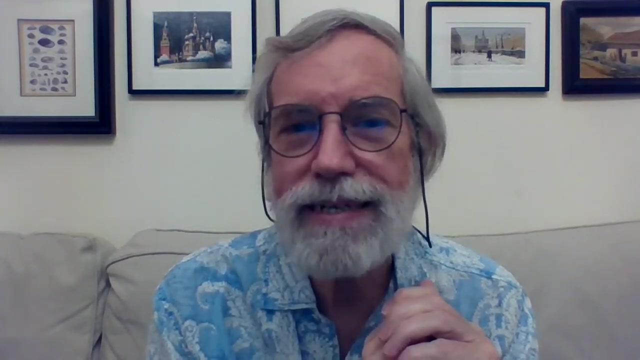 and those people are encouraged to work at home, only come into the office when they have to. Many of the meetings that used to be conducted face-to-face are now conducted remotely via Zoom or Teams or some other remote viewing mechanism. But yeah, it has impacted the work physically at. 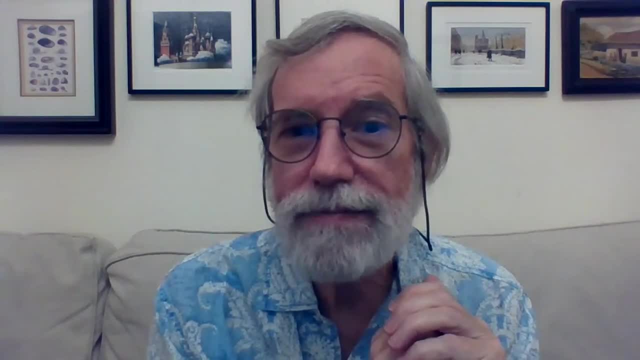 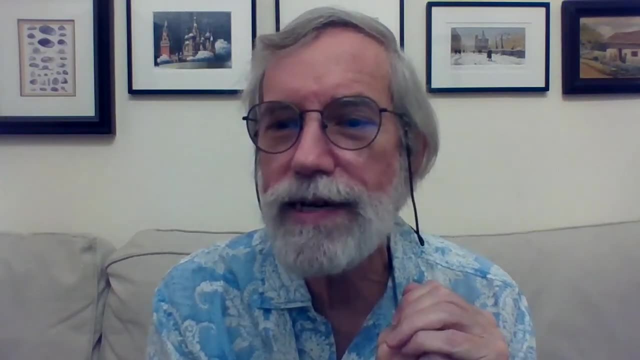 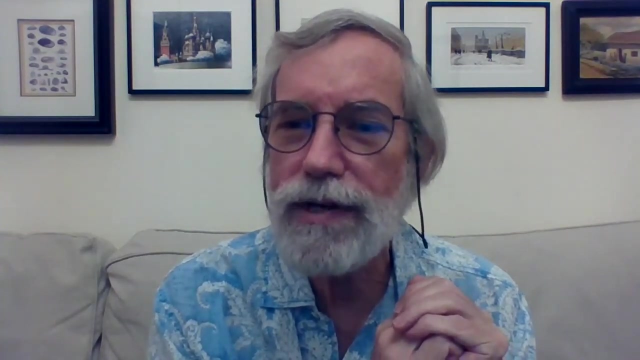 the agency, but they're still continuing on with their work. As far as me, retirees are no longer allowed into the Vienna International Center, so I can't go in there now because family members and visitors and retirees are not allowed access right now, only necessary staff. 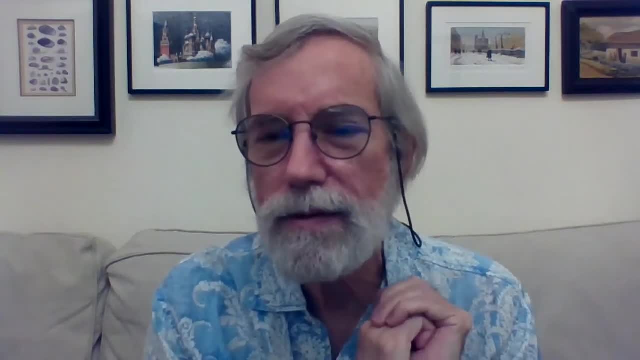 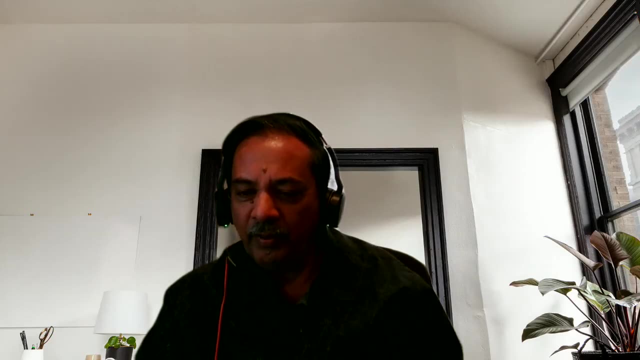 I see So the staff that's working in the field. second question also would be: can you talk about the climate change and the role of IAEA in nuclear power? What does the 2015 Paris Agreement say about that? Oh, I wish I could address that. 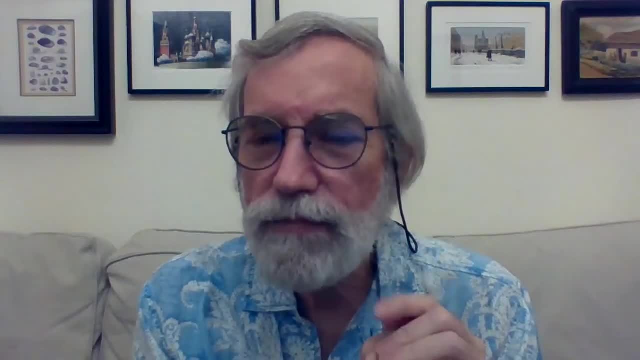 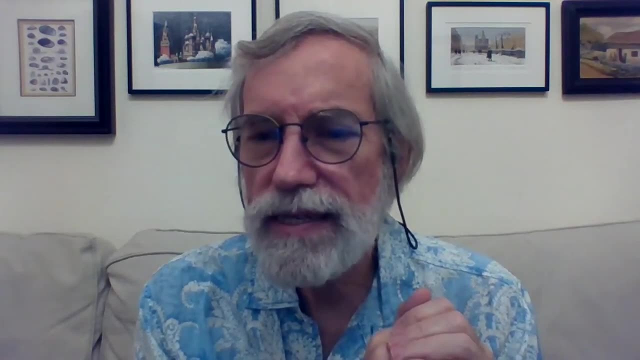 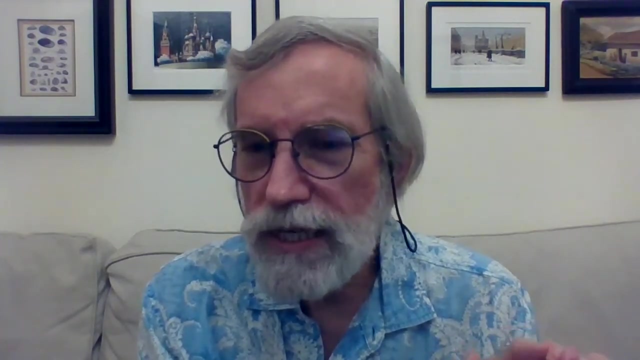 but I really don't have any information on that. All I can say about, from a climate change standpoint, one of the aspects of nuclear power plant development is they have to take into account those aspects of geology, geography and potential weather and external events. 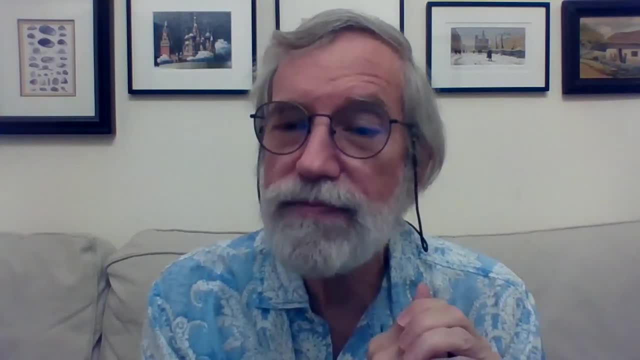 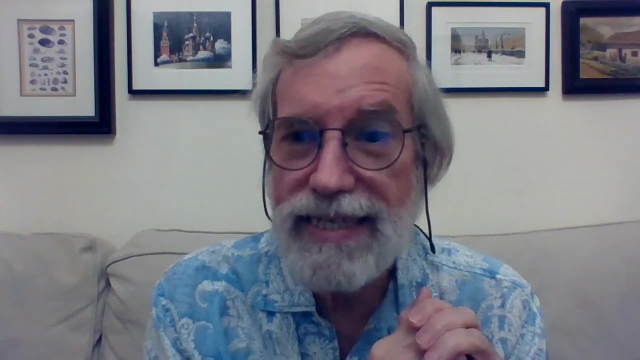 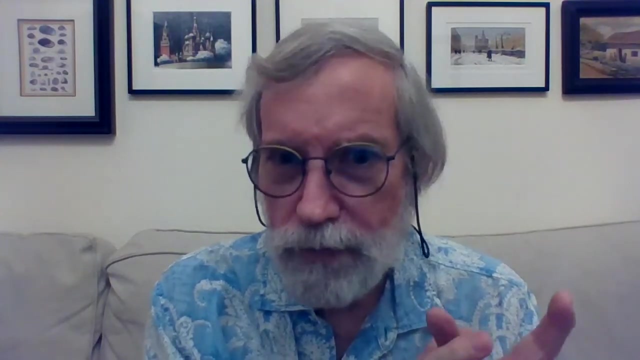 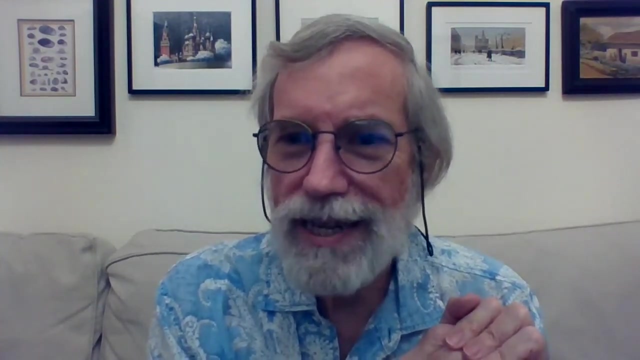 including flooding, storms and things like that. So those types of activities are required to be conducted or to be evaluated in the development of nuclear power plant- siting and things like that. So those activities are considered as part of the normal activity in developing a nuclear power program. But as far as the specific Paris Climate Accord, 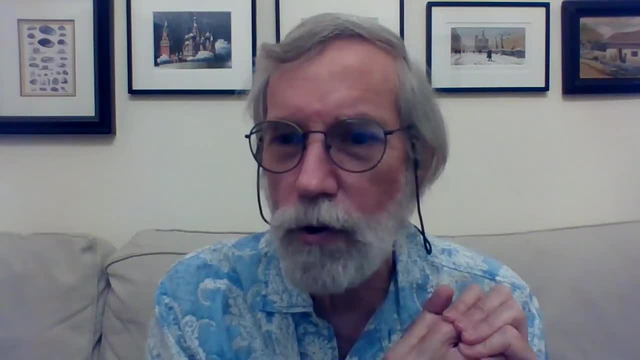 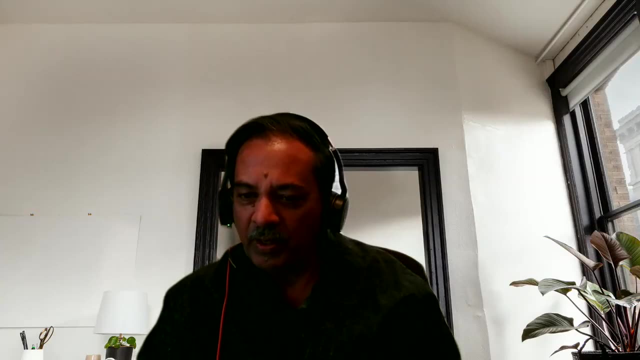 I'm not sure how that's taken into account specifically, or even if it is, I see. Okay, Now I think I overlooked. there are more questions coming in, Let's see. This is from Andrew. Thank you, Mr Graves. What is your educational background? Is it nuclear engineering? 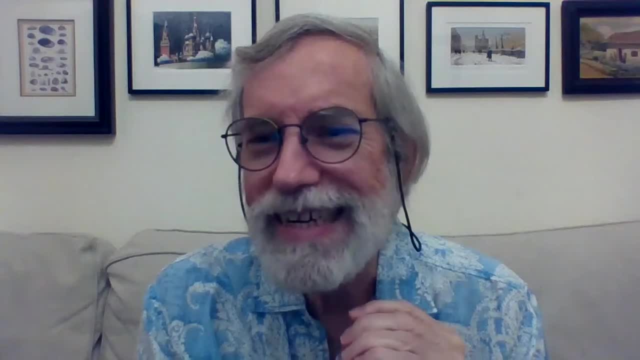 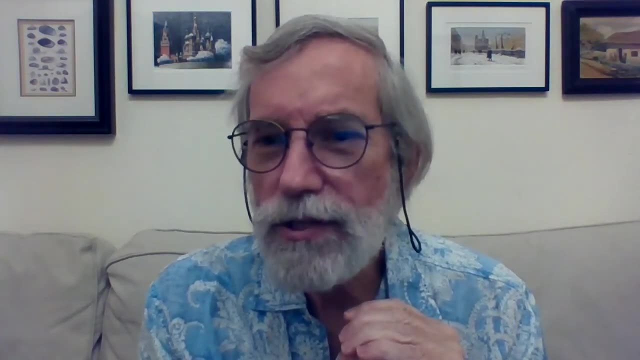 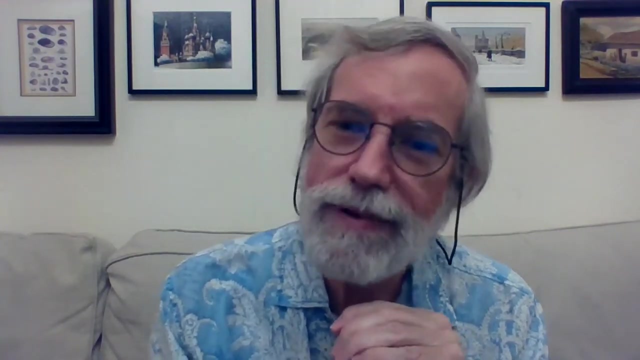 Actually my degree is nuclear engineering technology. I consider it like nuclear engineering light, But yes, I just have a bachelor's degree And basically what allowed me to get into IAEA was not only the degree but the experience that I have because I've been in the nuclear business. 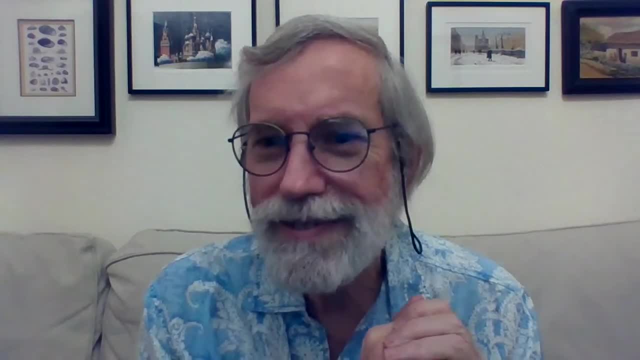 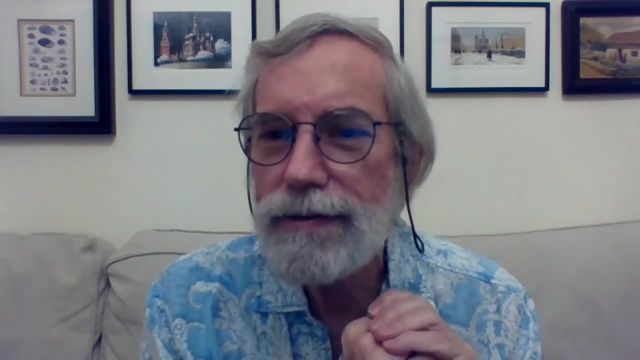 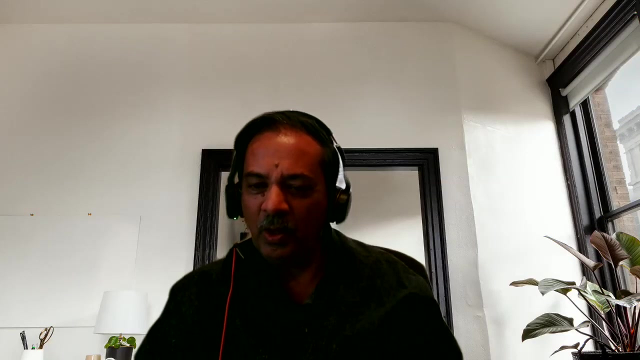 the nuclear field for 40 years. So the experience, I think, weighed much more heavily than than the educational background, I see. And so there was another interesting question. This is from Eric, And Eric is asking: is what sub were you on? I'm assuming the submarine he's talking about. 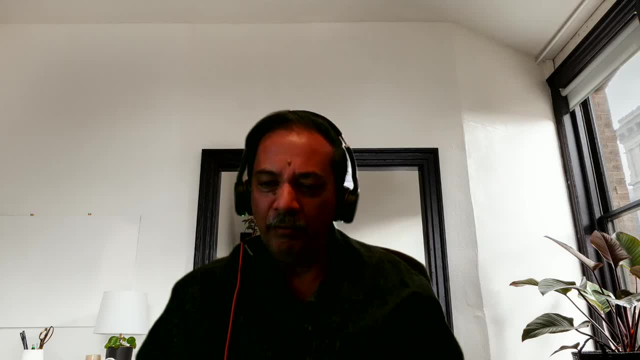 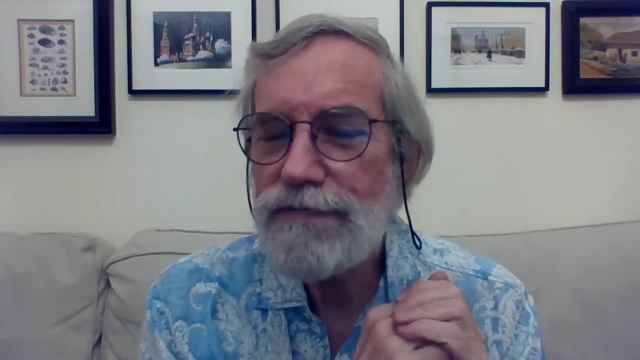 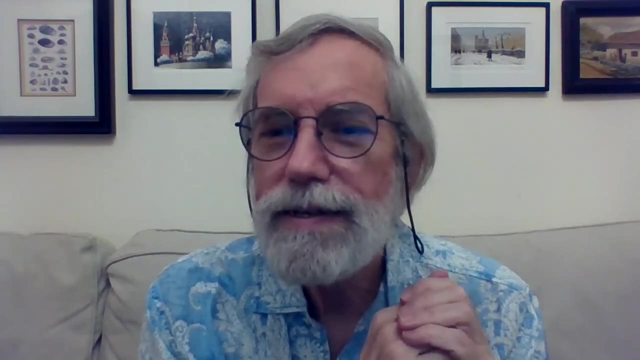 Oh, what was the question again, What sub were you on? Oh, what submarine was I on? Oh, the SSBN 658, the USS Mariano G Vallejo. Yes, It was a fleet ballistic missile submarine back in the. 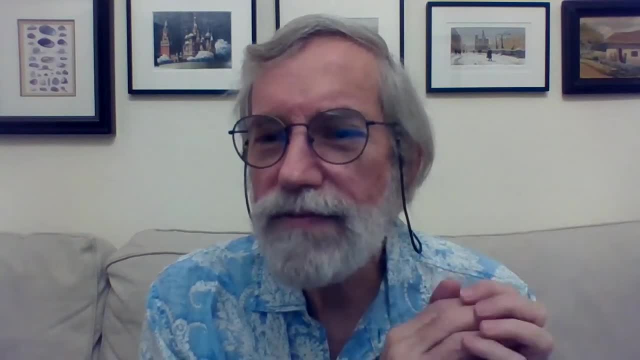 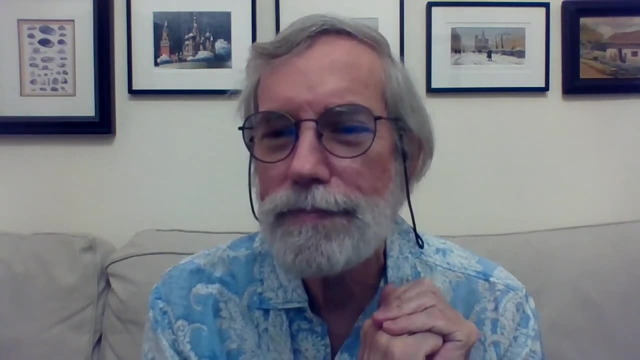 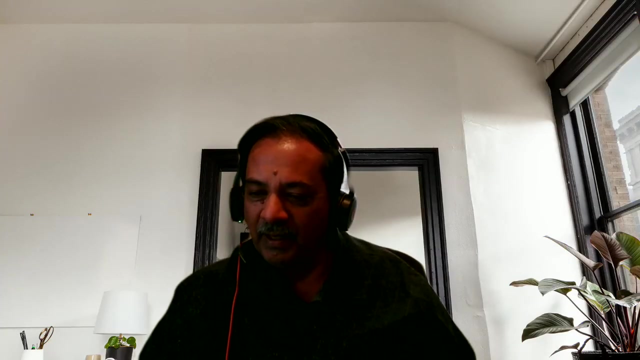 I was on it back in the 70s but it's out of commission now. It's scrap iron now it's been decommissioned and cut up, I see. So those are the questions coming from our students. Let's see if there is any other questions. 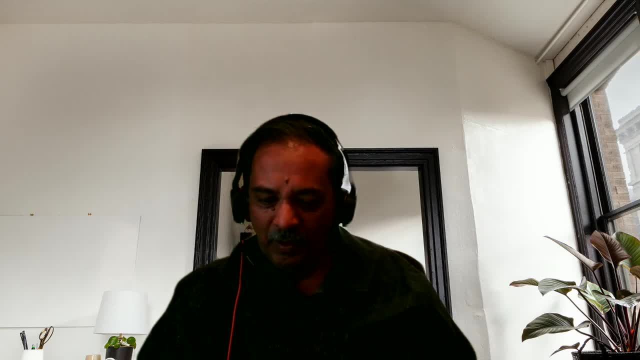 I don't see it. Here's the question from Zach Dr Kabar. Do you see it? Okay, And I'm not sure I'm not seeing it in the chat box. Okay, do you mind if I read it? 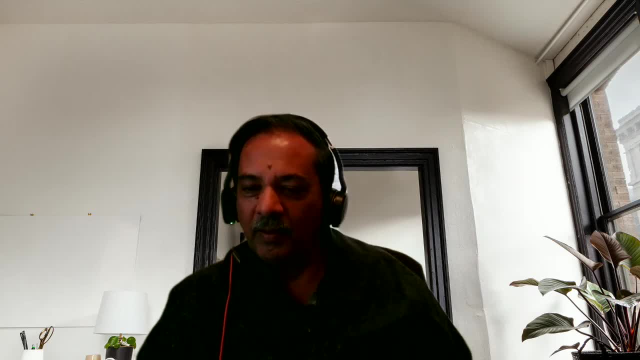 Absolutely okay. yeah, Okay, this is from Zach. He says, first of all, he's very jealous of the view that you have there in Vienna. It's not quite the same here in Arlington, as we all know. Secondly, what are some of the regulatory challenges? 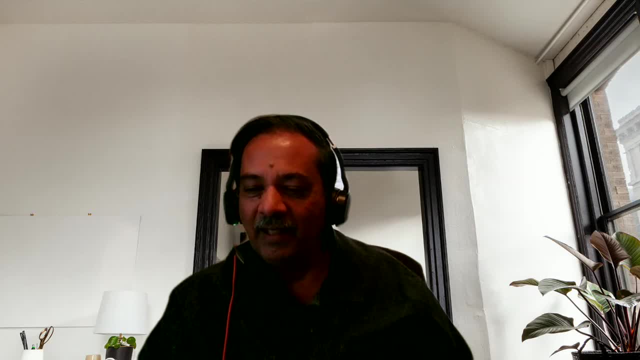 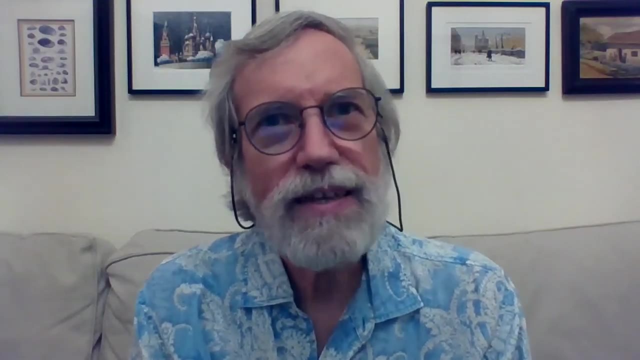 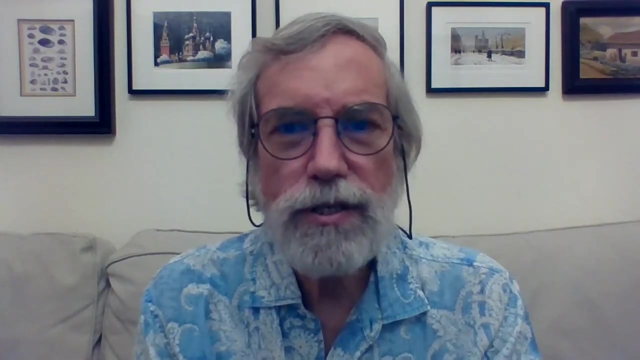 that the IAEA and the NRC face as, hopefully, gen three plus and gen four nuclear reactors become a reality. Yeah, some of the regulatory challenges we saw were very, I guess, have been longstanding and similar, especially for newcomer countries, countries that are just interested. in getting into nuclear power. Many of them don't have a very well developed regulatory infrastructure in their country. Some of these countries are, I'll say, poor countries. So not a lot of money. The governments don't have a lot of money. to spend on regulatory infrastructure. They're interested in nuclear power. Let's see how do I say this. They run into the challenge where the government typically gets involved in funding the development of the nuclear power plant as well as the development of nuclear power. so 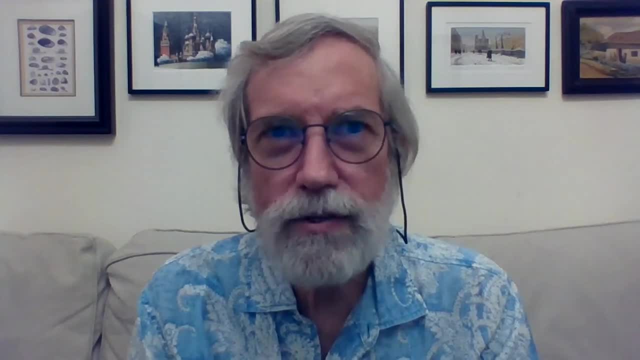 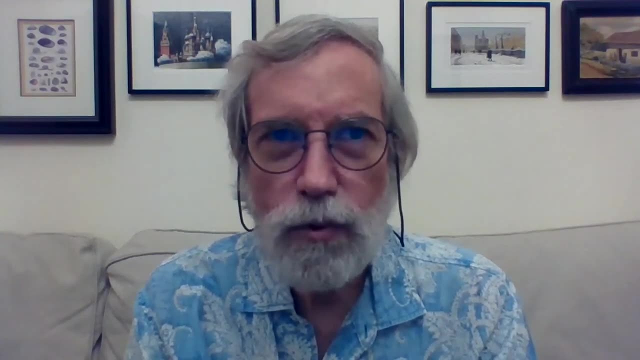 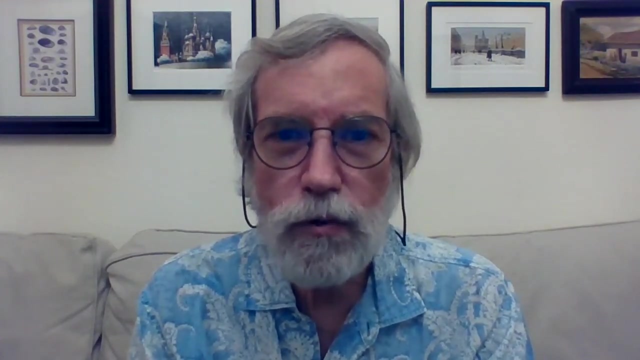 as well as being tasked with developing the regulatory infrastructure for that same industry, which tends to put them in the environment. the US was in back in the 50s and 60s with the Atomic Energy Commission. One of the things we strongly encourage them to do is to make sure that their regulator is independent of 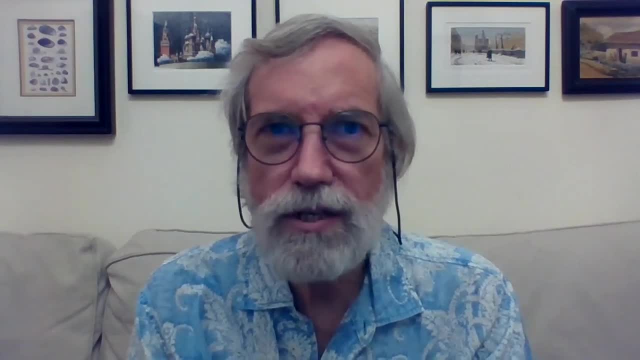 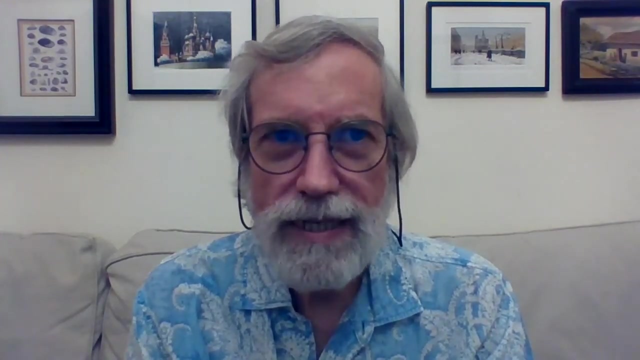 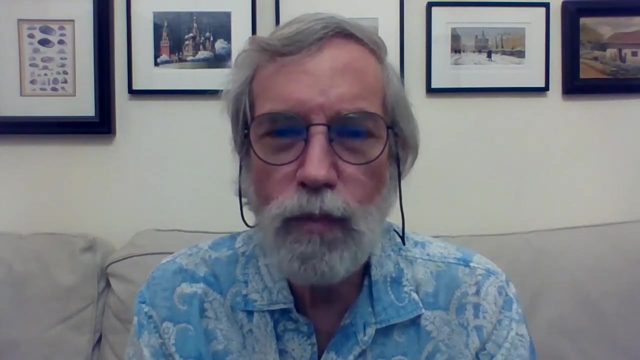 the operator, the operating organizations, such that they can provide independent safety oversight and regulation, and that is a continuing challenge with many member states. Another interesting thing that we saw coming up was an example would be the Convention on Nuclear Safety, which more or less commits member states to following IAEA safety standards and 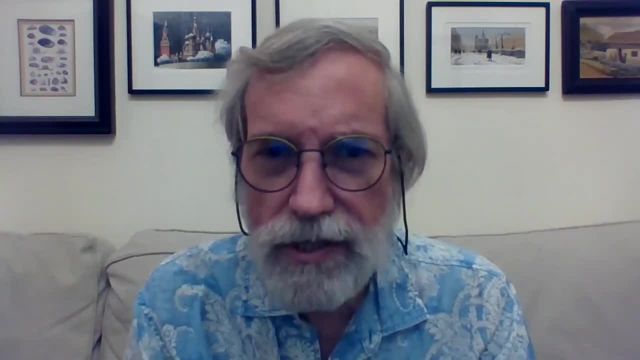 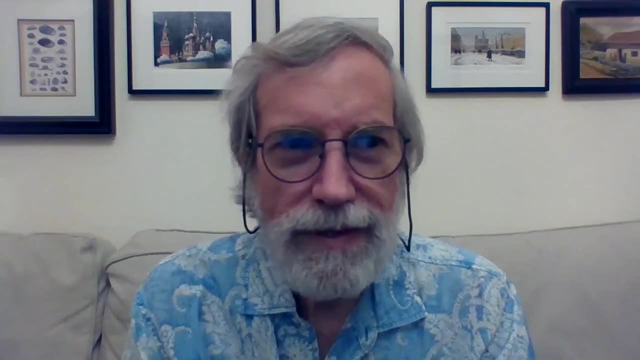 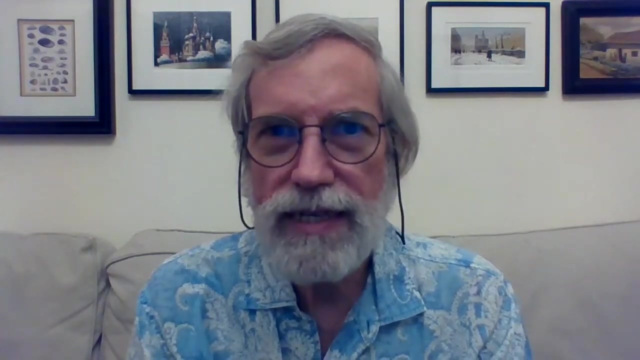 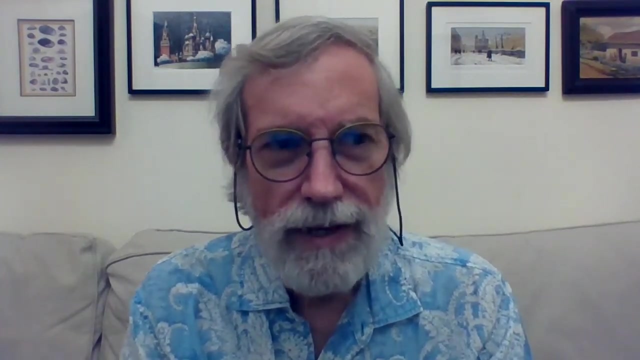 all those documents is the development of the floating reactors. At least one country has developed mobile floating reactors, which the question comes up: how does that fit into the regulatory framework for land-based reactors? So that was another interesting concept. A lot of the 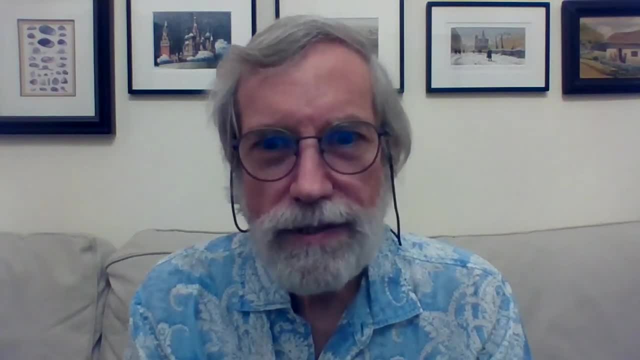 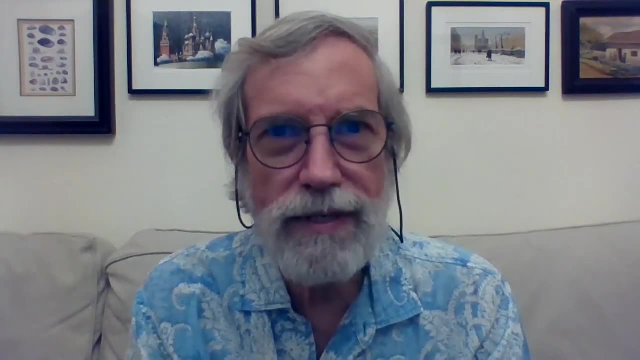 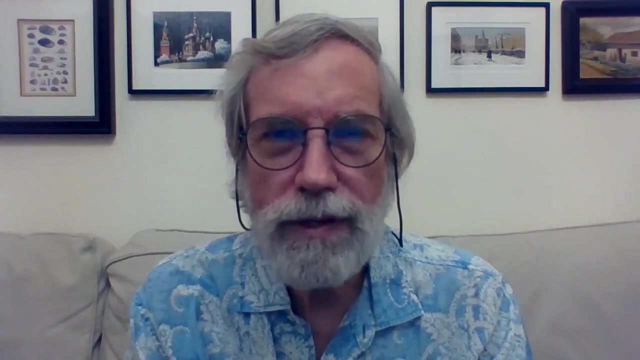 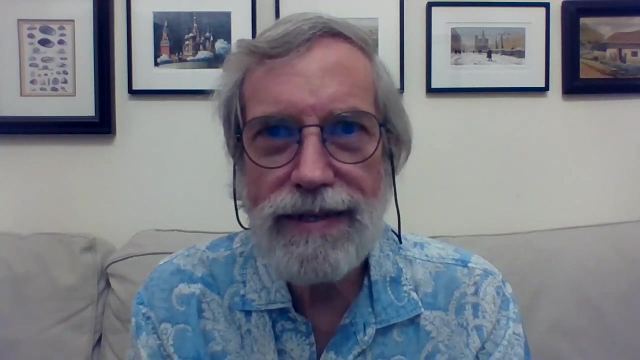 regulations are based in light water technology. so, as new designs come up, not only with Gen 3, Gen 4 plants, but with new innovative reactors that use something other than light water- for moderation or for cooling, the regulatory framework needs to look to make sure that. 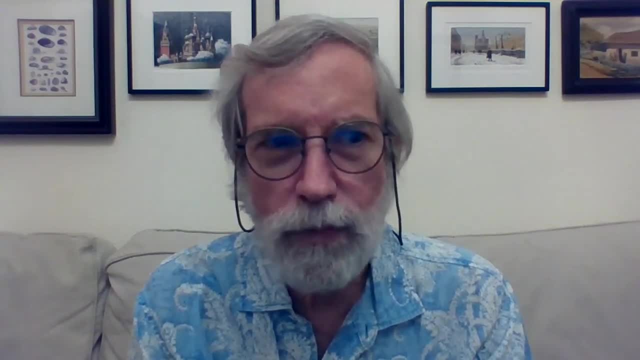 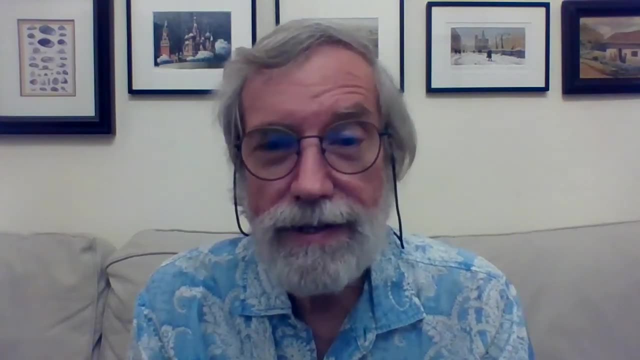 those activities are covered or captured by the existing framework and, if not, modified accordingly. So those are some of the challenges faced. So, as a follow-up, this is coming up. So, as a follow-up, this is coming up. So, as a follow-up, this is coming up. 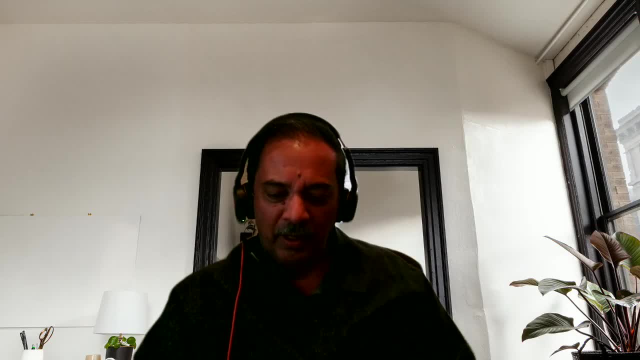 from me, David. So in US I know that we have NRC that provides the regulatory oversight. okay, And US is also a member country. So is there any kind of overlap or a conflict between IAEA safety standards and what NRC prescribes? As a matter of fact, not really The IAEA provides. 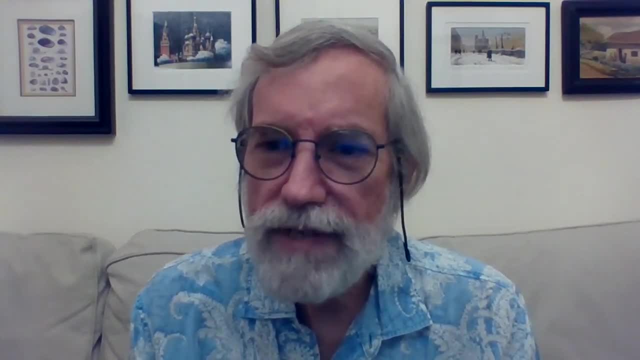 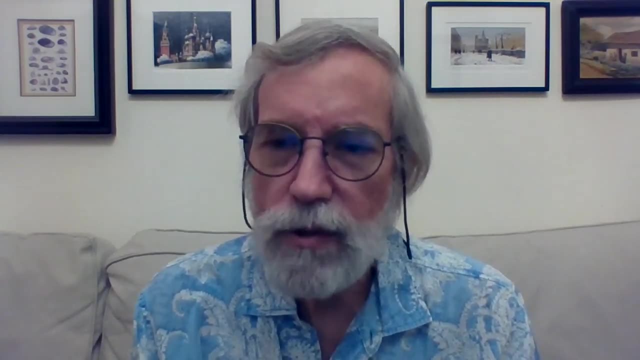 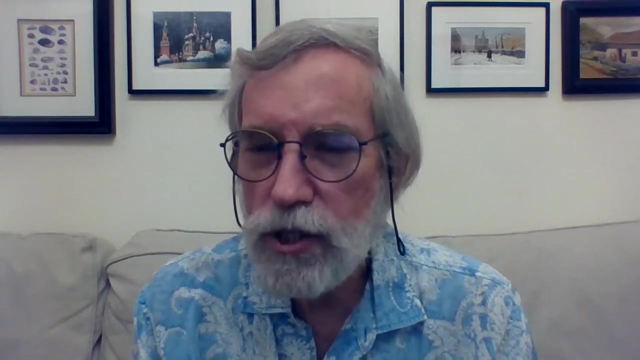 the guidance via the safety requirements and safety standards, but it doesn't have to be word for word. The member state can take that guidance, take the requirements and the guides and they can implement them in their country, basically however they choose. But ideally, 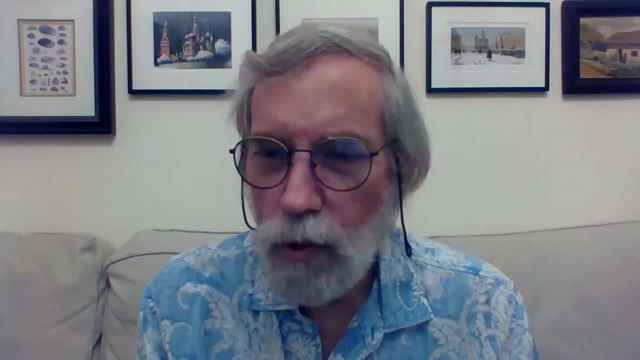 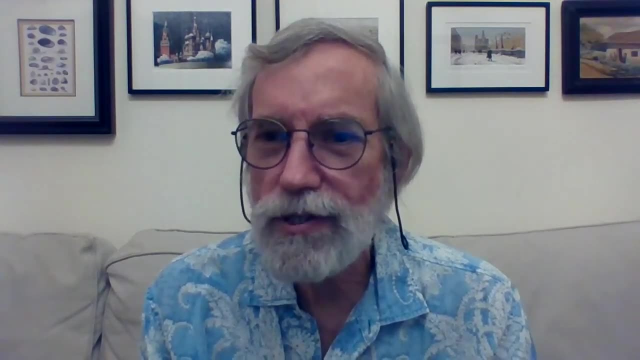 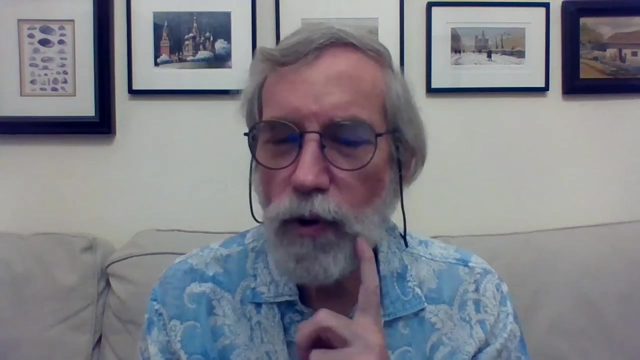 you know, they would still take the concept or the requirement and just use it within their regulatory framework, as long as the, as long as the, the safety function gets implemented, the mechanism by which they do it is okay. So for NRC standpoint they would. they would take the IAEA safety standards and then, as long 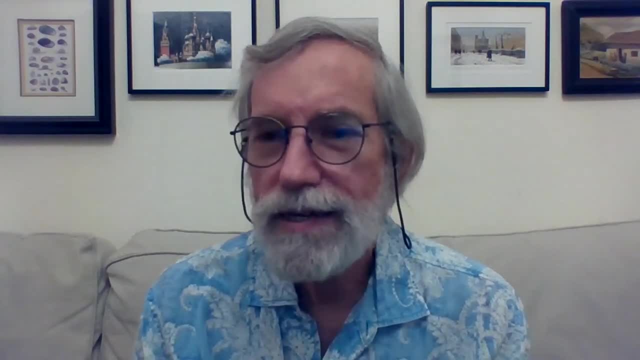 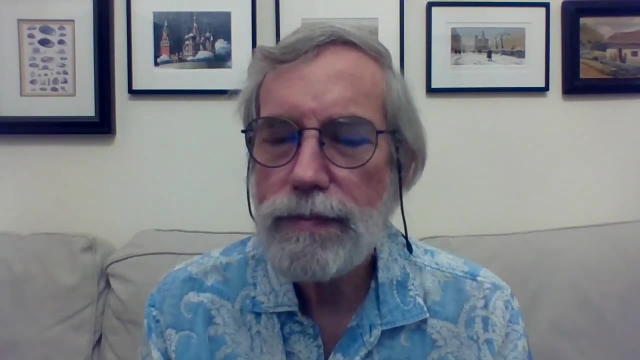 as the safety standard is implemented in the NRC regulations, that would be satisfactory. I mean, that's fine, I see. So I think with that and with the one hour window closing in now, I think we should be done with question and answer. 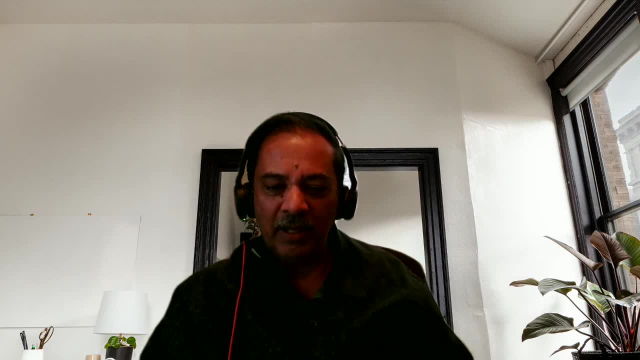 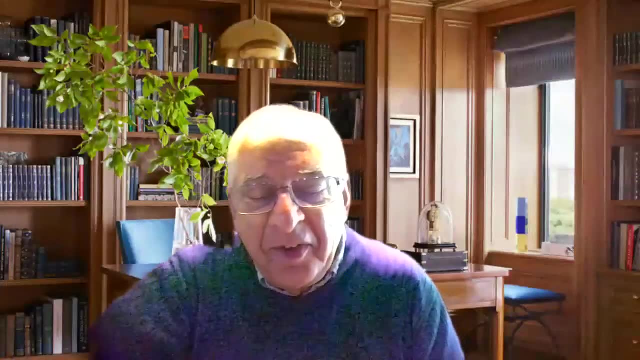 So, but last part, I think Dr Kanerangvi. he has a important announcement to make And if he has any questions, David, I'm just going to turn it over to him. Thank you, Thank you, Thank you, David. 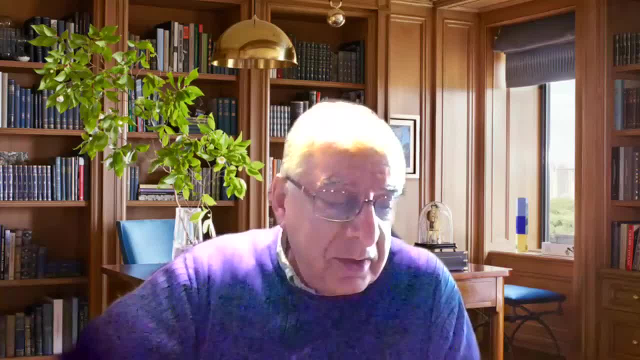 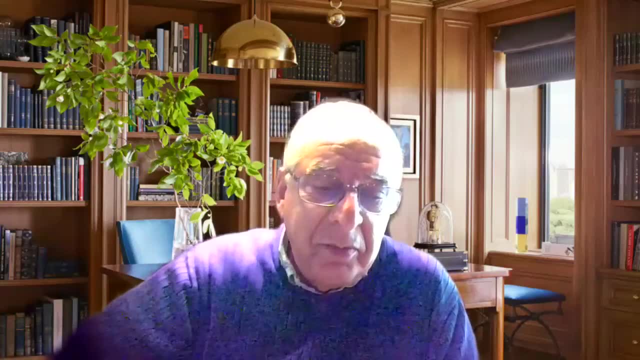 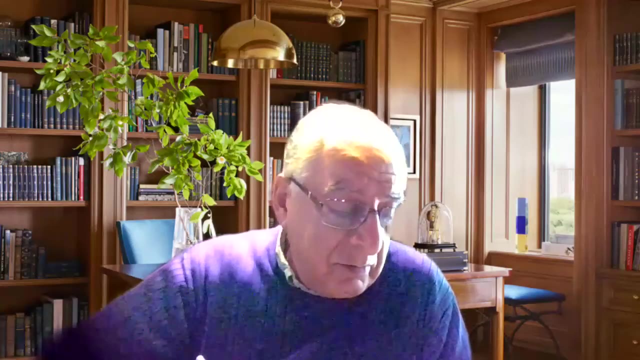 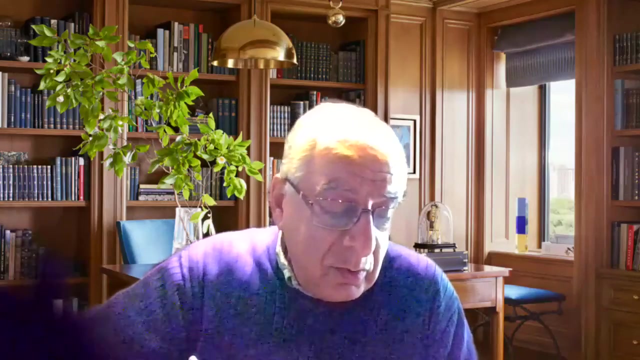 Dr Mary Danzig-Gore. she's the president of ANS- American Nuclear Society. She will be presenting a seminar multi-student ANS sections within the UT system on Tuesday March 23rd at 9.30 to 10.30 central time.